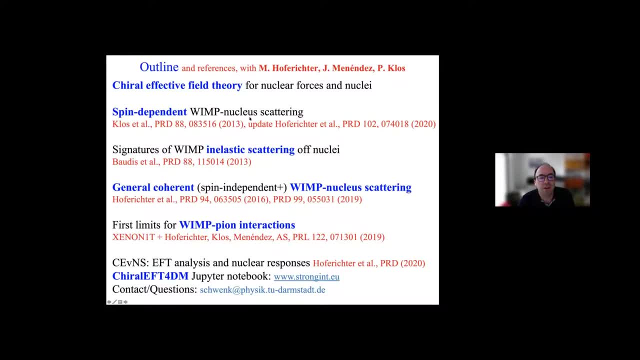 WIMP nuclear scattering- And here's the key paper here- Close 2013.. And there's an update in our 2020 paper, Thank you. And then I would like to discuss also a very interesting channel in the inelastic scattering, where nuclei are excited from the ground state, which is maybe too difficult to detect. but 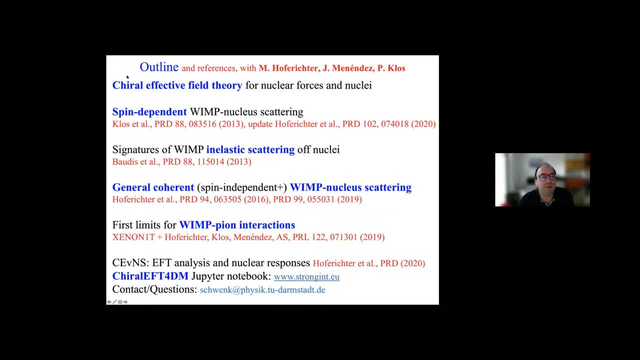 very, very interesting if it can be realized, And this is what we will do today And tomorrow. we switch to a more, more, let's say a broader, picture of WIMPs coupling to nuclei and discuss all possible coherent. so spin-independent is one of them, but all. 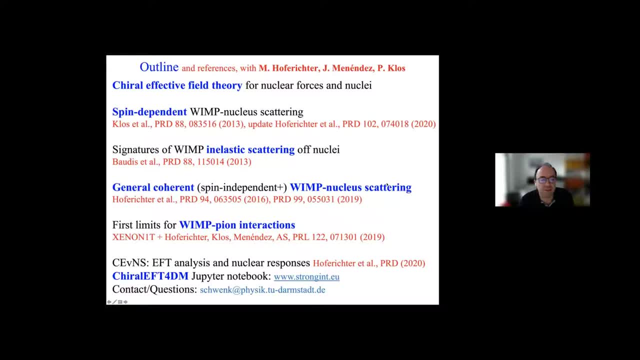 possible coherent WIMP nuclear scattering channels. And I point you to these two papers, in particular the most recent ones, And also want to show how that has been used to provide first limits on WIMP-Pion interactions from the Xenon-1-TAN collaboration. Then let me 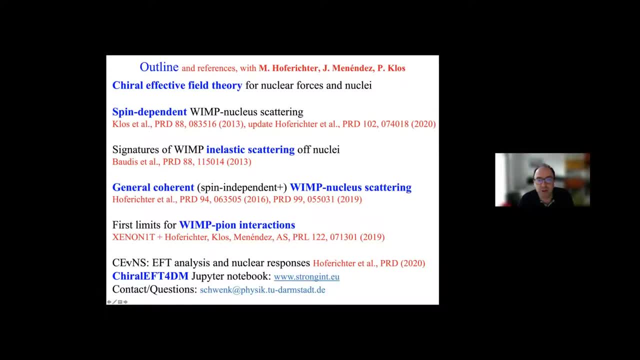 make some advertisement for an additional work, recent work here, which is that paper where also there was a spin-dependent update. Maybe we also looked at coherent elastic neutrino nuclear scattering, also using the same current EFT framework and nuclear responses. So if 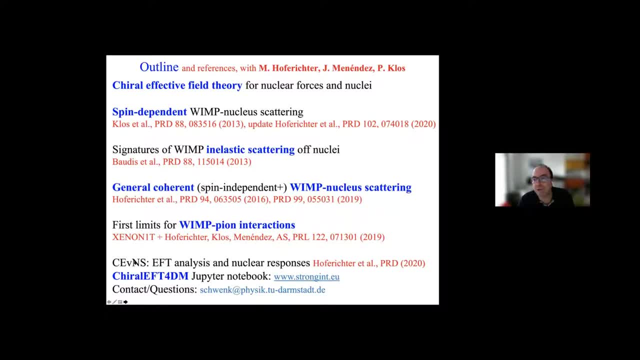 you're interested in using consistent neutrino scattering rates to the dark matter nuclear scattering rates. this is covered by this paper. And then we wrote a Jupiter notebook which is available On our group's website, the Kyron EFT40M, which is able to calculate all these responses. 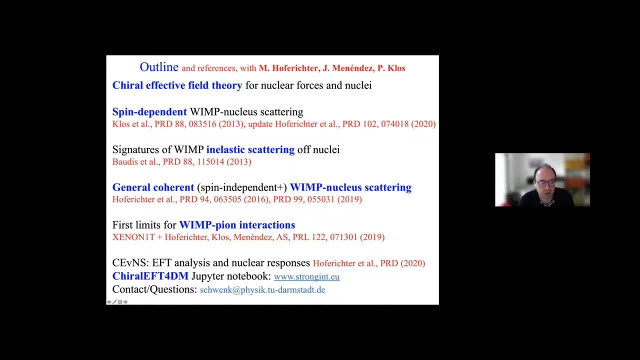 and from these also calculate WIMP, coil spectra and so on. And finally, if you have any questions outside of the school or after the school, please feel free to send me an email to my email address, which is here. Okay, Let me start with the first topic, which is basically: 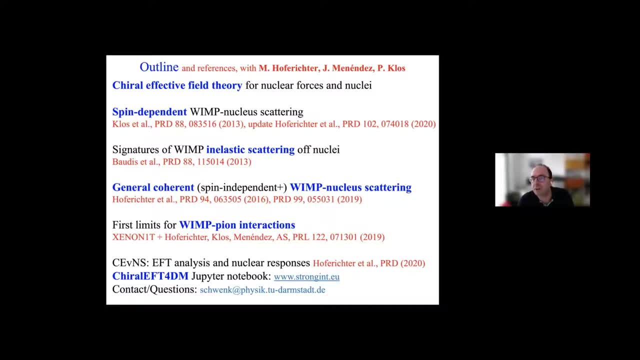 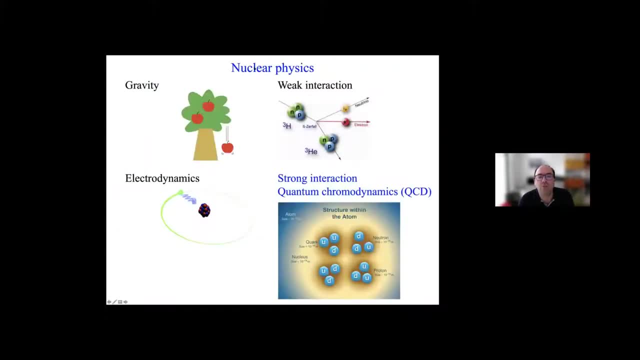 a quick introduction to modern nuclear physics, which I think is important Because you will have to rely on nuclear physics for some aspects of dark matter, direct detection. So nuclear physics concerns primarily the strong interaction, one of the four fundamental interactions of nature, And it's, as you know, governed by QCD, which is the theory. 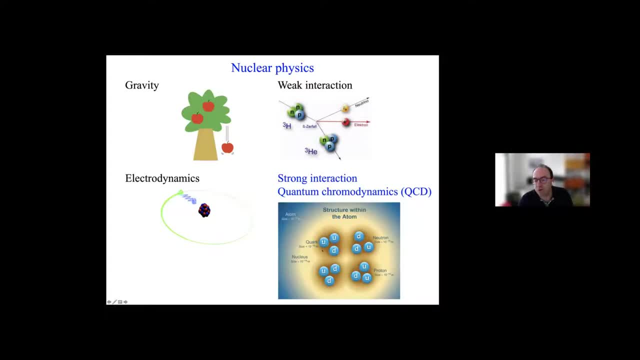 of quarks and gluons, which binds quarks and gluons into heterons, like neutrons, protons, and they themselves form nuclei, bind to neutrons. And then we also have the theory of quarks and gluons, which binds quarks and gluons. 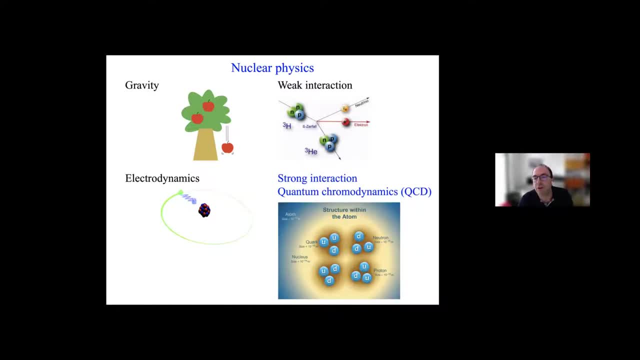 into heterons, like neutrons protons, and they themselves form nuclei. bind to neutrons, like neutrons protons, and they themselves form nuclei. but actually all of the other four fundamental interactions of nature, the weak interaction, obviously, electrodynamics. 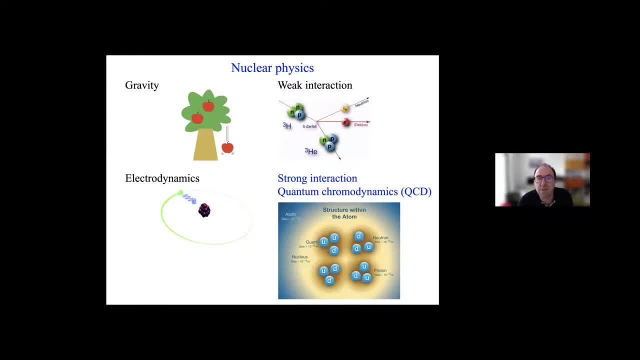 and also gravity are very close to nuclear physics. So in nuclear physics we are, at the level here of the energy budget of the universe, interested in the strong interaction which is basically what gives the mass of ordinary matter, the 5% of ordinary matter in the universe. 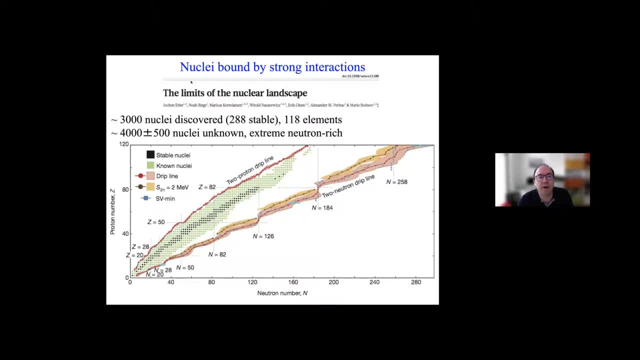 Okay, So a big quick overview of which nuclei are bound by the strong interaction. This picture here of the alpha particle, already helium-4.. And you are of course all familiar with stable nuclei because they are served as targets for dark matter, direct detection. But just 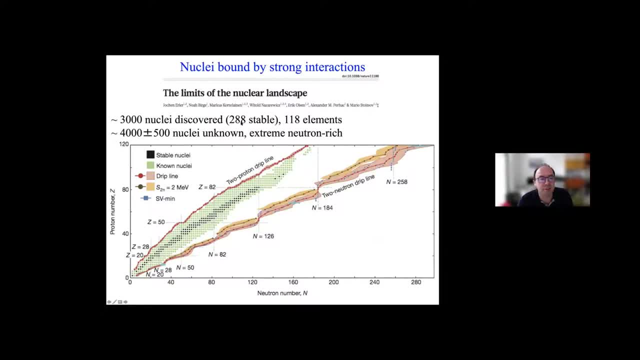 to tell you that they are not just about 300 stable nuclei, but there are factor X1, maybe 3000 nuclei that have been discovered. You're all in Greece, Okay. Most of them are, of course, unstable. They beta decay, for example. And this paper here. 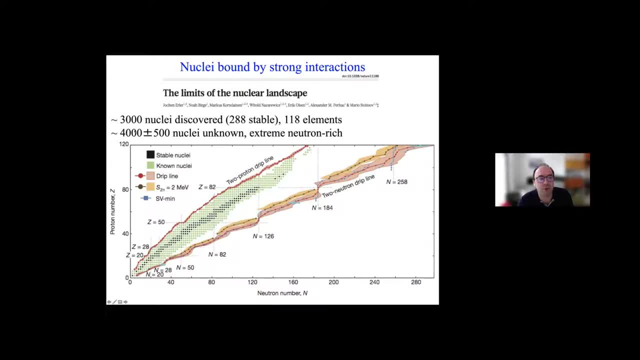 predicts that in fact there are at least as many more nuclei that are held together by the strong interaction. And you can see here that if you look at nuclei in the nuclear chart, where they are arranged as a function of proton and neutron, number all of these. 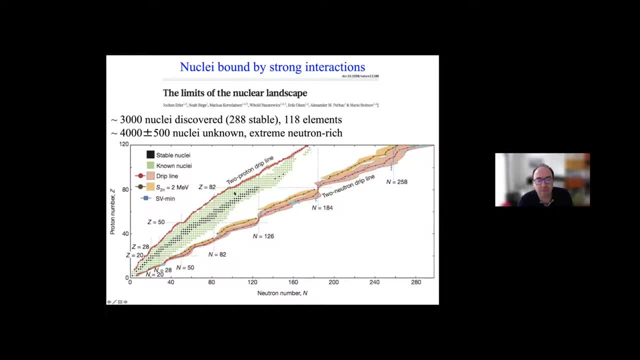 unknown nuclei here lie between the green points that have been discovered and the so-called neutron drip line, which is the heaviest possible neutron-rich nuclei for a given element. Okay, So all of this? in all of this white space, there are bound nuclei by the strong interaction. 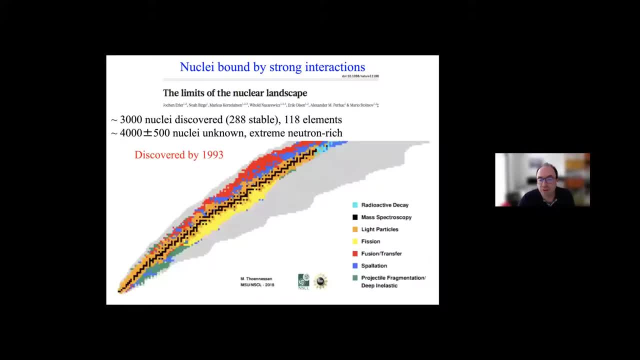 that exists, Just to tell you that this has been actually something that's really taken off in the last 20, 30 years Over. here you can see the state Okay In 1993, which was 25 years ago, compared to this last compilation of where all nuclei 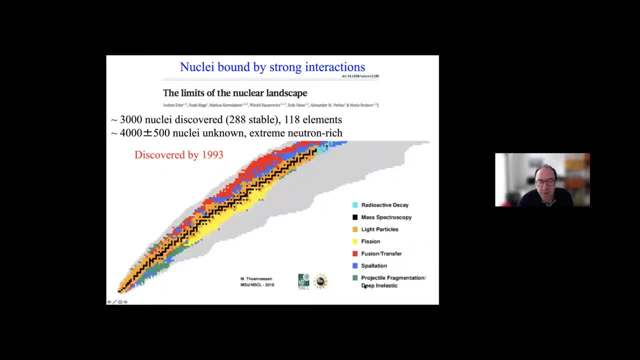 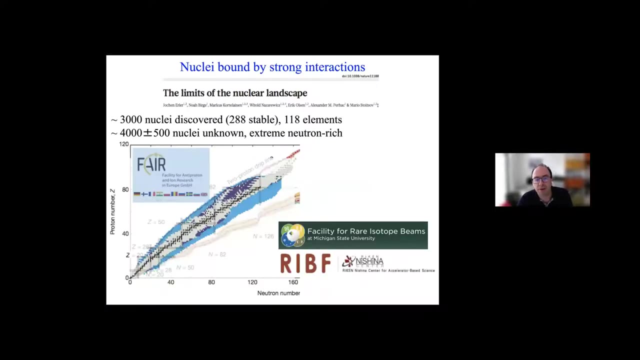 have been discovered through various channels here And if you look at the last compilation then you can see there have been many neutron-rich nuclei that have been synthesized in the lab and discovered in the last 25 years, And in fact there are three large facilities that are either operating at RIKEN in Japan. 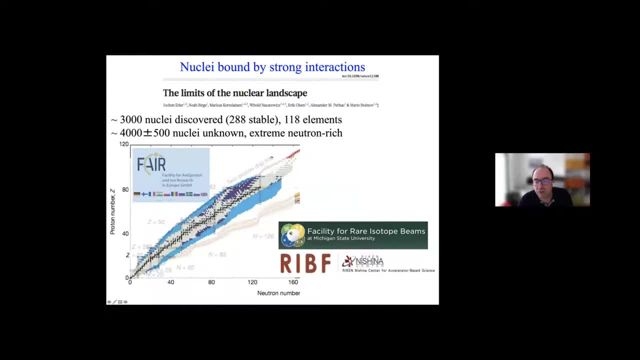 under construction and close to operating at F, the facility for rare isotope beams at MSU. and under construction and set to operate in a few years, FAIR, the facility for antipotent ion research in Darmstadt. And the reason that the nuclear physicists are so excited about this is because this: 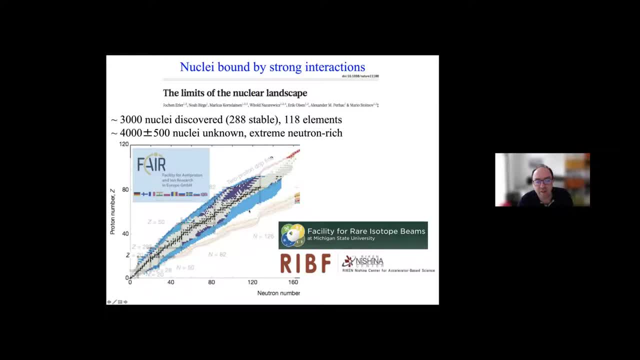 will basically, in some regions, fill in half of the territory that is unexplored of these exotic neutron-rich nuclei. Okay, And so you can see that this has also spurred the nuclear theorists to really refine methods that we use to describe nuclei. And that's very important to you because you want to. 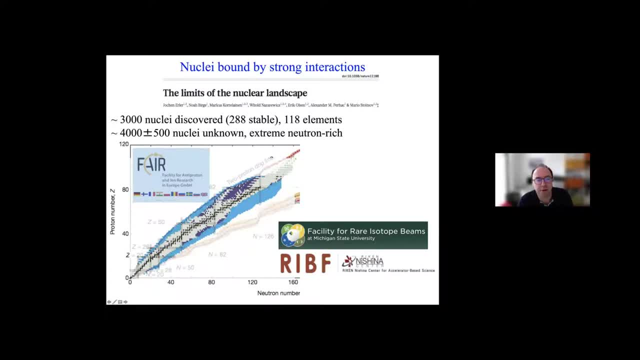 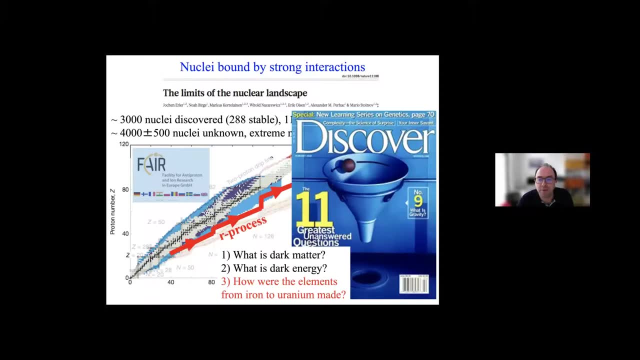 use accurate nuclear physics information for dark matter direct detection. So let me give you a little bit of a broader view why this is so important, To quote from this Discover magazine, which formulated the 11 greatest unanswered questions. Okay, For their top three, they basically took the energy budget pie chart and turned it. 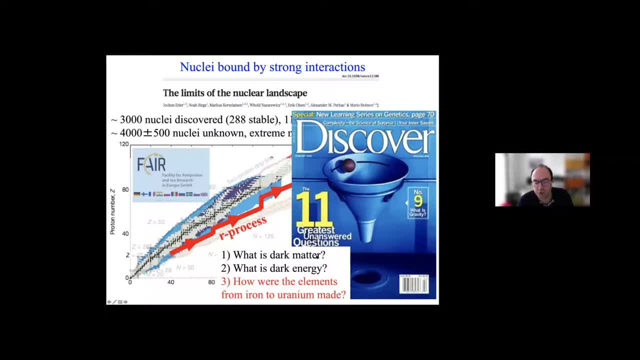 into questions: What is dark matter? Your school, What is dark energy? And in nuclear physics, we're after the question: how were the heavy elements from iron to uranium made? These were made through a process that is called the R process, which is a way of synthesizing. 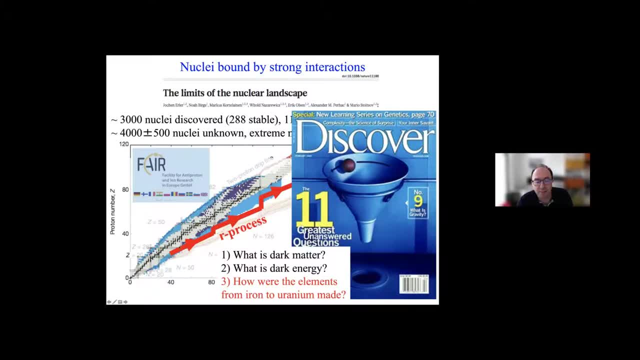 nuclei along this essentially red line here By capturing many neutrons rapidly- that's why it's called R for rapid neutron capture process- before they eventually beta decay back. And I just want to show you how that works And notice that this runs through basically a huge region that is experimentally unexplored. 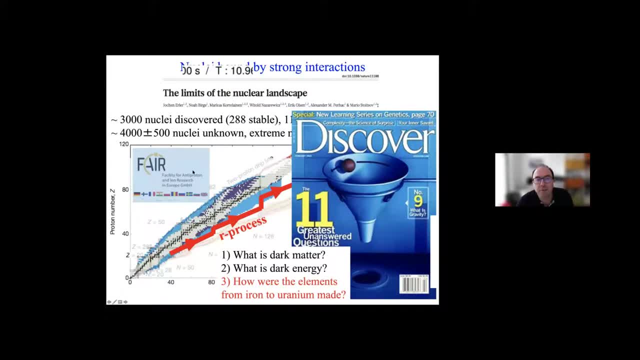 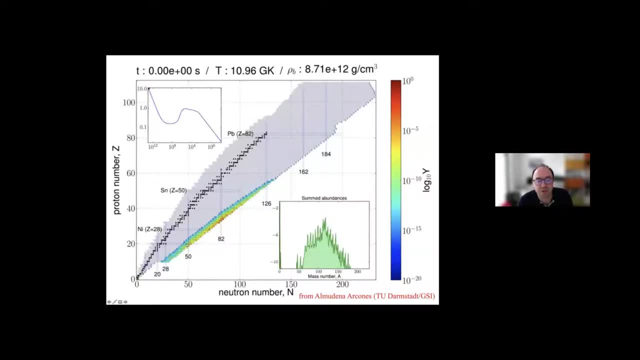 and will be explored by future facilities. Let me show you here in a movie of how this happens. So we start in an astrophysical environment with some nuclei that are already existing here around- iron group nuclei here in red- And then, if the movie runs, we have to wait. 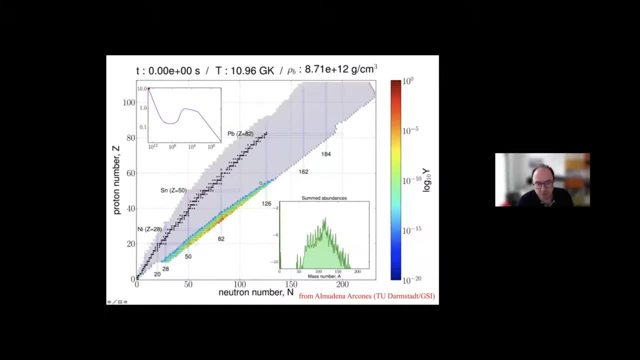 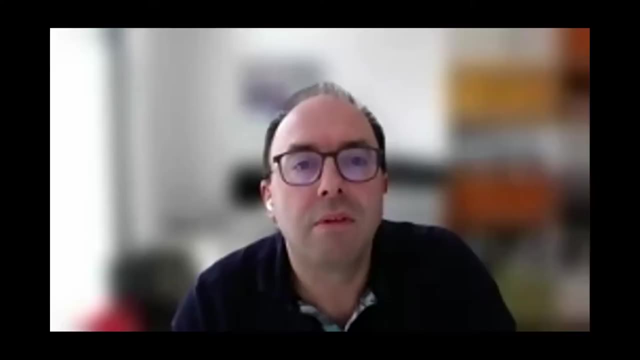 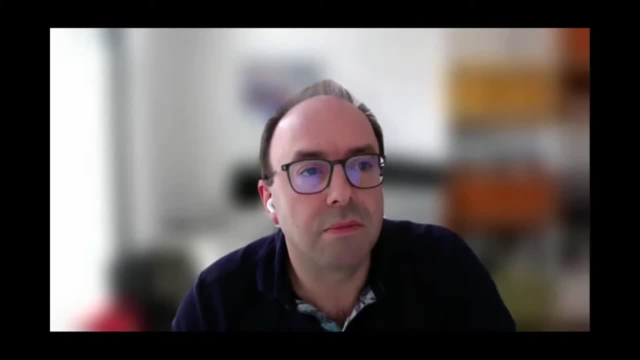 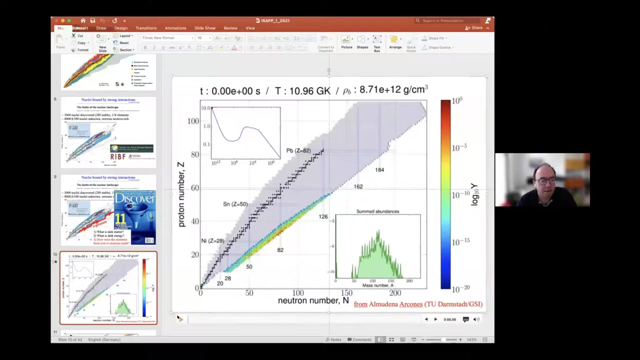 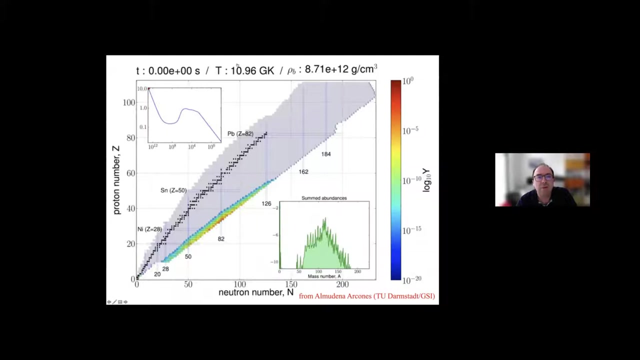 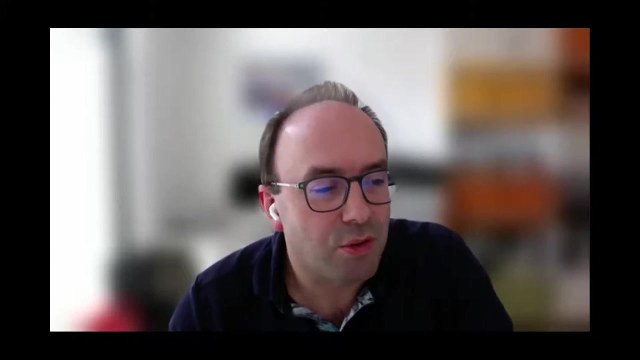 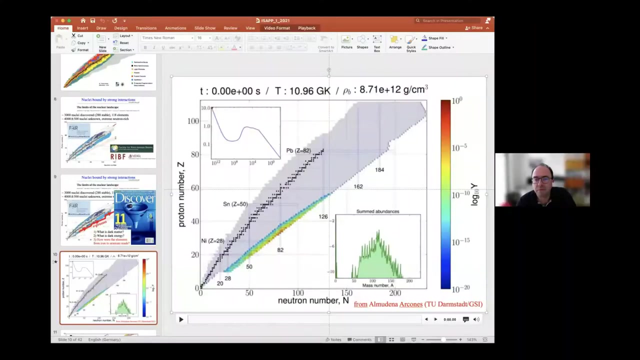 Okay, Okay, Okay, Okay, Okay, Let me do the movie here. let me try again this way, And then my computer doesn't like me anymore. okay, never mind, we still skip the movie. you can ask me in the exercise session. you basically synthesize all the heavy elements along this our process path up here and 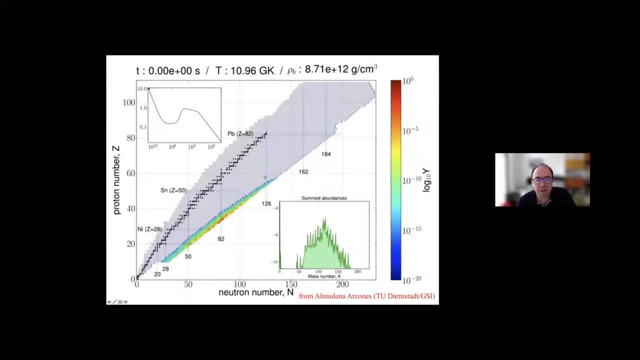 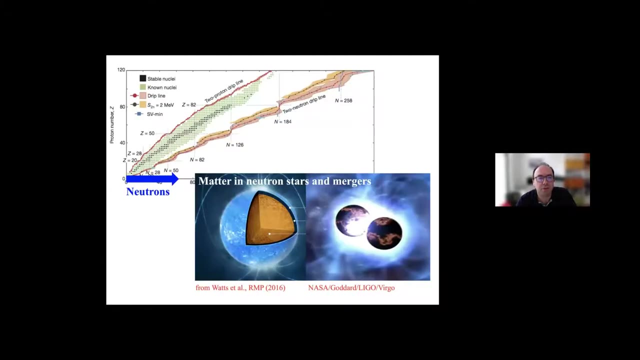 then these synthesized, freshly synthesized neutron-rich nuclei beta decay back to over here and form the abundances observed in the solar system. i think this file is just so large for zoom, that's the problem. okay, and so basically you have a synthesis path that goes along. here you need very neutron-rich environments, and so that happens either in. 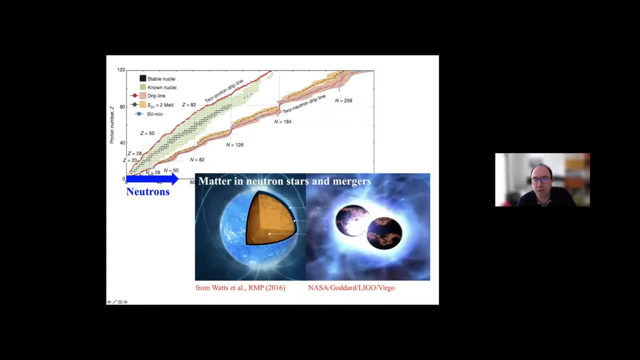 phenomena occurring in neutron stars, or you have very neutron-rich environments, and so that happens either in phenomena occurring in neutron stars, or you have very neutron-rich environments, and so that happens either in phenomena occurring in neutron stars or neutron star mergers and from this, decay of freshly synthesized neutron-rich nuclei. 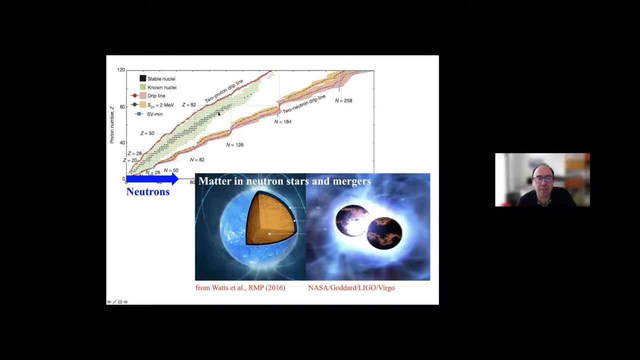 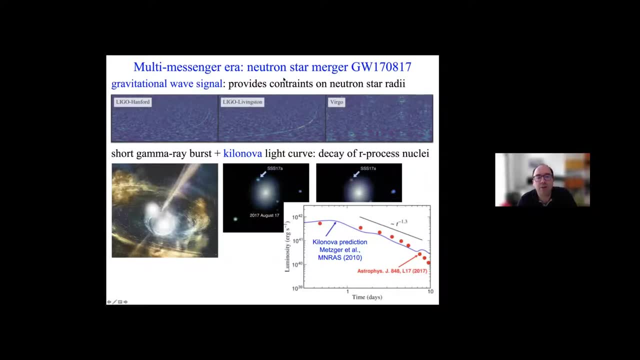 from this beta decay back, one can get energy gain and this can be observed. and i just wonder, since you have also in your network a gravitational wave school, then of course you know that there has been, have been neutron star mergers that were observed, the first one in august 17th. 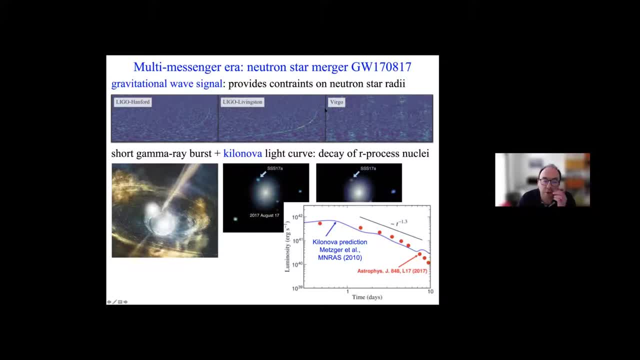 2017, with this inspire signal here at ligo, and also after this merger, there was not only a short gamma ray burst observed, but also kilonova, so a faint supernova which turned from blue to red over short time, and you can see here the observations from this kilonova, which are in blue. sorry, 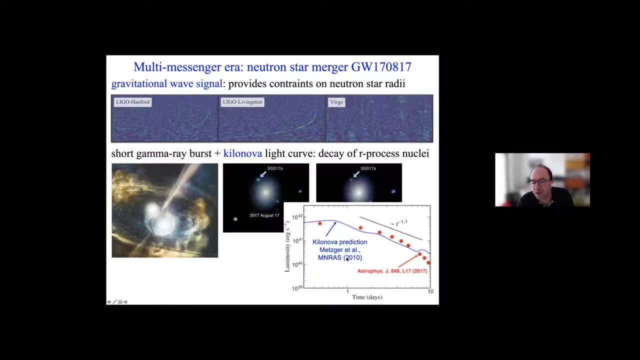 the in red points and blue to the earlier prediction here by Metzger and collaborators, which was a prediction which relied on the nuclear physics input by nuclear physics colleagues here in Darmstadt, Arcones and Martinez-Pinedo, So actually the nuclear physics that we want to tackle. 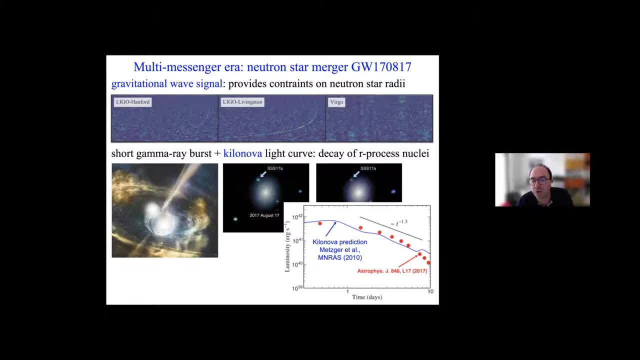 and the nuclear structure that we want to tackle plays not only a role for nuclear structure or for decays, for weak decays or, for you, for dark matter, nuclear scattering, but it also triggers all these astrophysical light curves and it plays a key role for neutron stars. 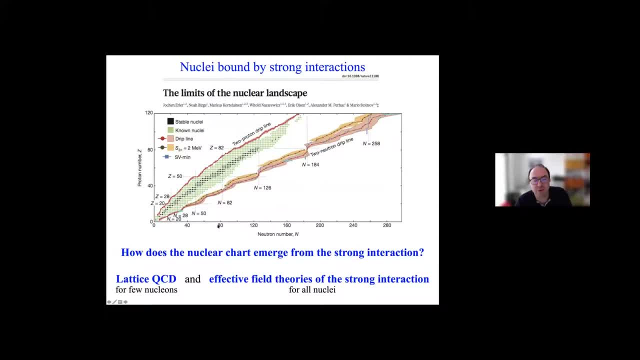 Okay, so let me come back to what we're really interested in, And we want to describe nuclei for dark matter, direct detection- and so we want to ask the question: well, how can we describe nuclei based on the theory of QCD? 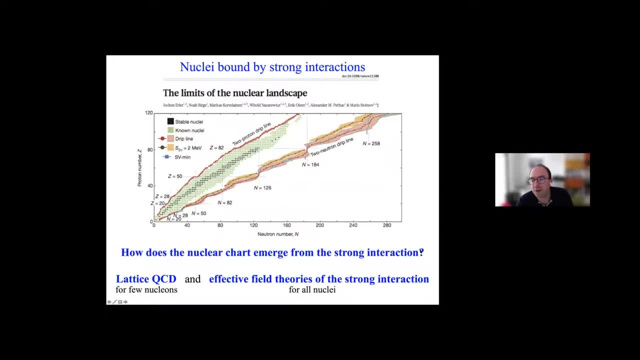 And there's essentially two paths forward. One is the real, direct way, namely: So take the theory of quarks and gluon QCD and put it on space-time grid and simulate it using powerful lattice simulations. However, because of the sign problem, 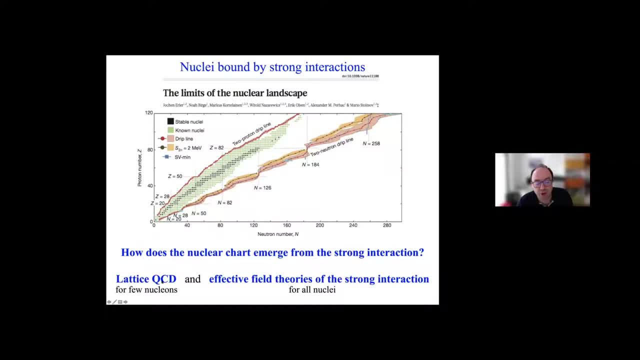 and because of large signal-to-noise ratio, this is not possible at the moment, except for systems of few nucleons, which is basically here. And since you are interested in nuclei as heavy as xenon, that's not useful for you, So you can use the theory of quarks and gluon. 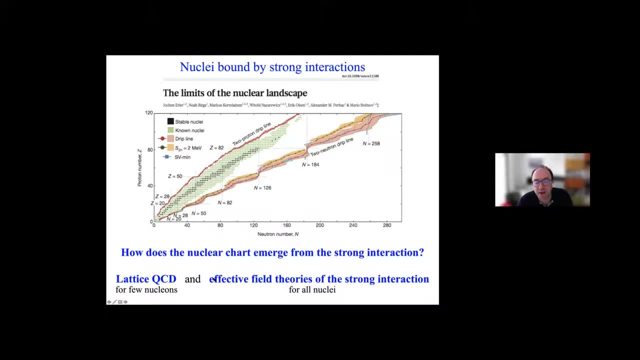 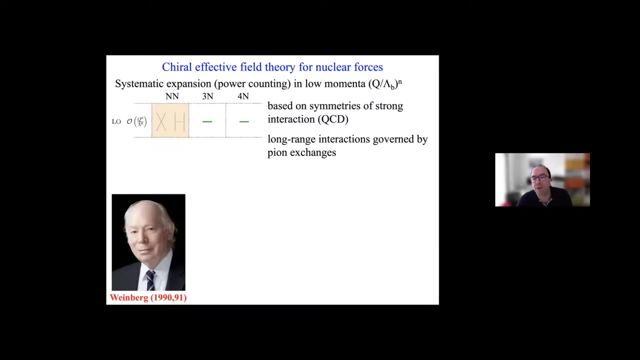 to describe the dark matter direct detection. Instead we use to describe the nuclear chart and nuclei, not QCD directly, but we use effective field theories of the strong interaction which have been used for many nuclei And in fact we think can be used for all nuclei. 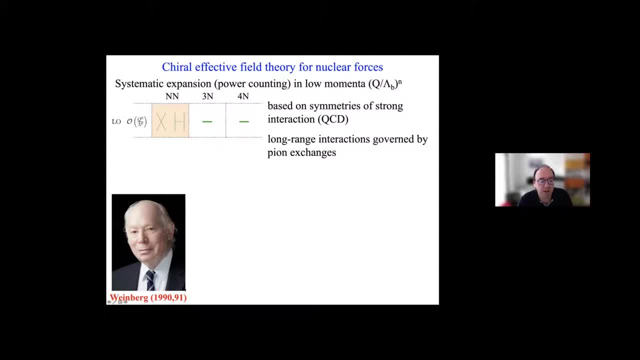 So what is the prime effective field theory that we use in nuclear physics? The prime effective field theory was introduced to nuclear physics 30 years ago by Steven Weinberg and it's called the general effective field theory. And here's the implementation used today. 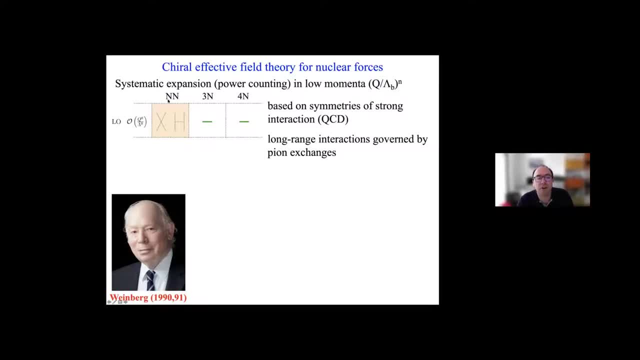 in its description of nuclear forces, meaning the interactions of nucleons, two nucleons, three nucleons, four nucleons in free space or inside a nucleus. And the effective field theory of Steven Weinberg basically writes down all possible type of interactions of protons and organizes them in a systematic expansion. 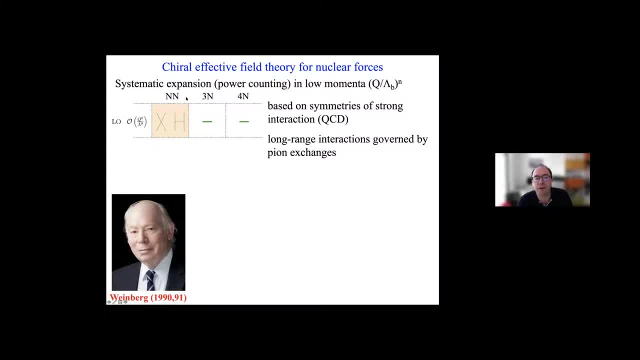 not in terms of the coupling constants, because in the strongly interacting theory none of the coupling constants are small, but in terms of momenta of the nucleons. So this is a diagram for two nucleons interacting at short distances, or two nucleons interacting 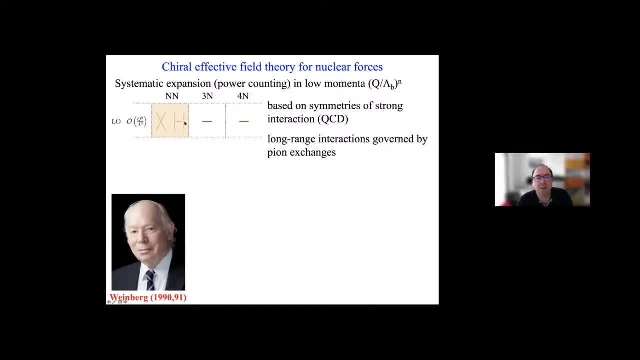 by exchanging a pion. And Weinberg predicted that if you're interested in the nucleons having low momenta, so low energy nuclear forces, then the dominant interaction, the leading interaction in this momentum expansion is given by having only two nucleon interactions. 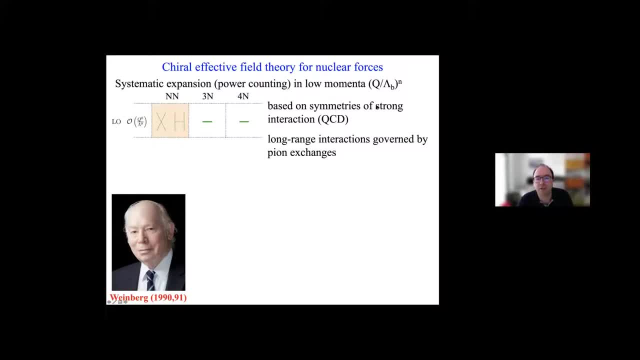 And he wrote down all possible type of interactions based on the symmetries of the fundamental theory of QCD, And the theory is called chiral effective field theory because it includes, as degrees of freedoms, as we discussed here, The nucleons and pions. 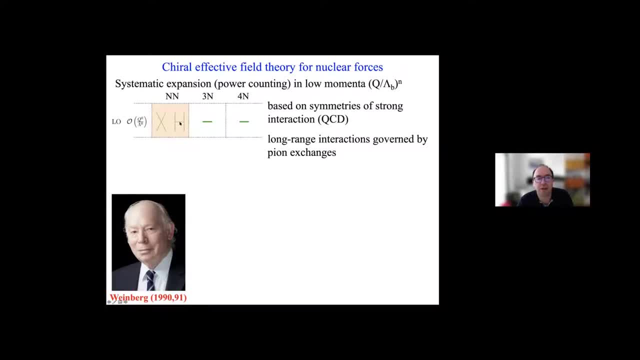 And because the pions are the Goldstone bosons of chiral symmetry breaking, we call this theory chiral effective field theory. So Weinberg predicted the leading order interactions are just two body interactions. Then, at next to leading order, so suppressed by two powers of momenta, Q there. 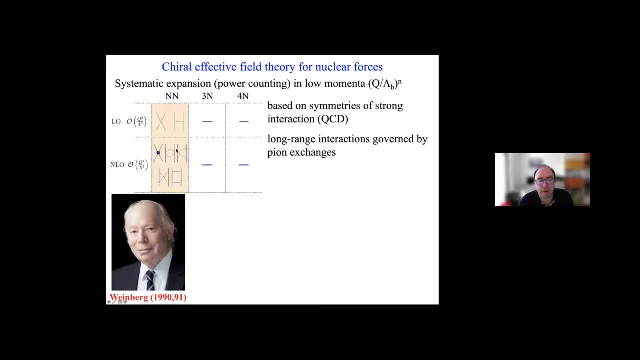 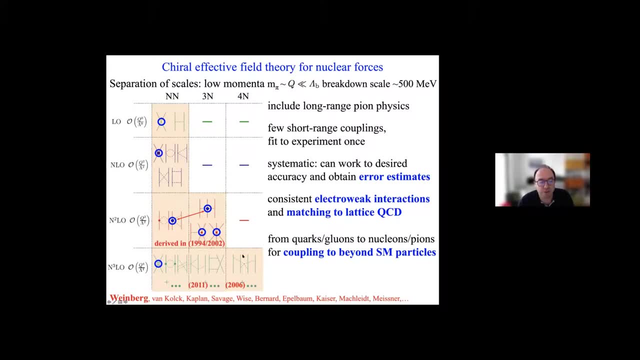 are corrections to the two body interaction And at the next order there are three body interactions And at higher order there can be even four body interactions, And you can see here that this field has been making steadily progress by deriving all these interaction contributions. 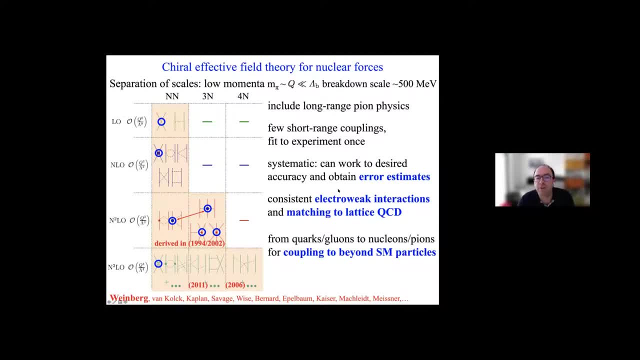 So what's the advantage of this effective field theory? The first advantage is that we include all the long range known pion physics explicitly. The second advantage is there's a whole bunch of short range couplings Which we don't introduce through a model. 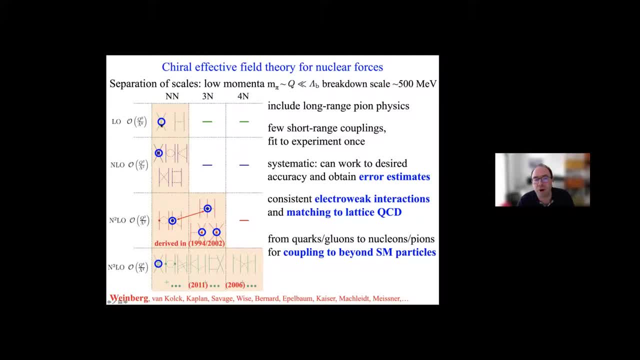 But these couplings, like in an effective field theory, are fit to experiment once. So we could fit these guys here to two body experiments, like two body scattering experiments, And the rest this could be fit to three body scattering experiments. So we have a few short range couplings, actually not many. 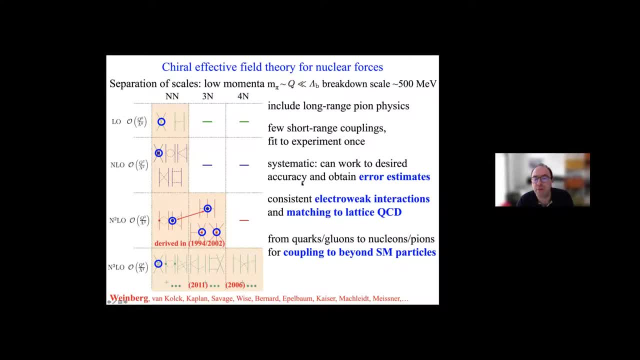 And there are some orders where there are no short range couplings at all, And they are fit to experiment, And so this is the first advantage, And then the second advantage is that we can actually do this experiment once, And so then, this nuclear chart that we discussed- 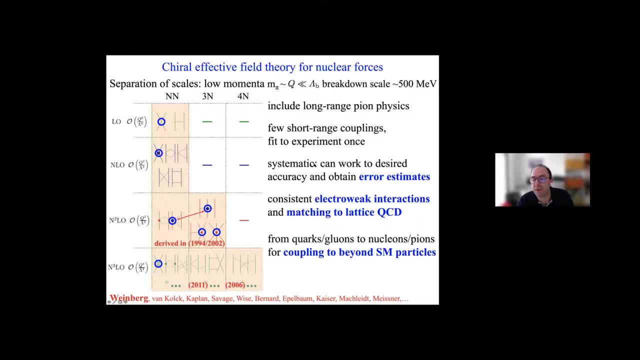 should come out without three parameters, without changing any couplings. It's a systematic effect field theory. We can work to a desired order up to NLO, up to N2LO And obtain uncertainty estimates from what's left out through the EFT convergence pattern. 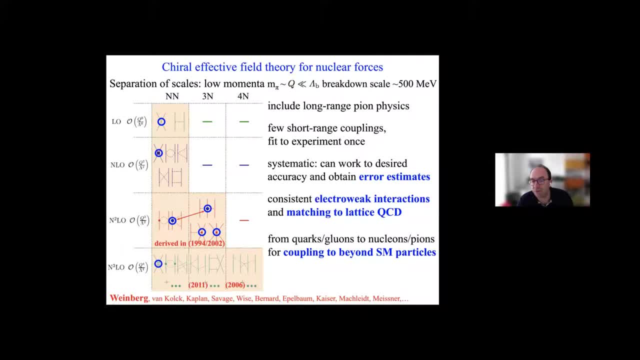 Because it's a field theory. we know how to do coupling interactions like to minimal substitution, just as in the standard model, except it's done at the level of the effective field theory. We also know how to match to lattice QCD. 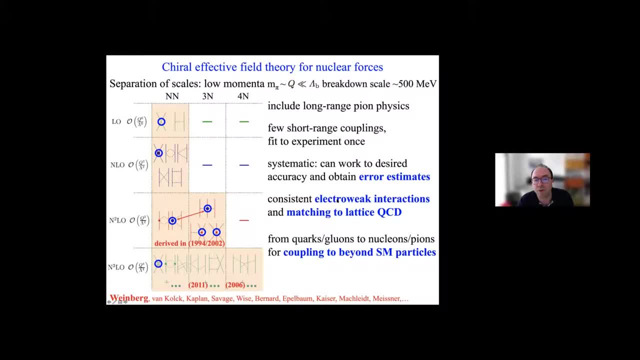 And we know how to not just couple to electromagnetic photons or weak bosons, but we know how to couple to any other probe that's outside of this theory, to any beyond standard model particles, in particular to any dark matter coupling channel. OK, So 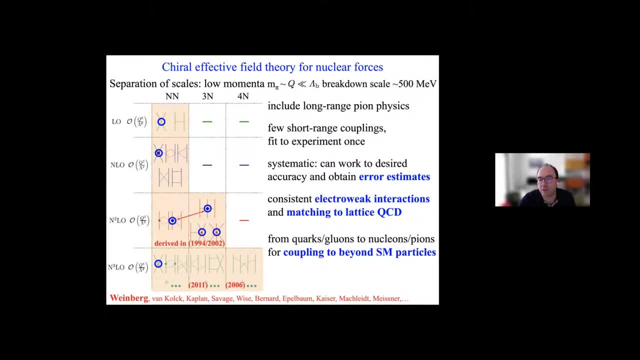 This is a systematic organization not just of the strong interactions in the nucleus but consistently of how the nucleons in the nucleus interact with any external probe And for every one of these there's such a systematic organization principle, There's a leading order interaction of the nucleons. 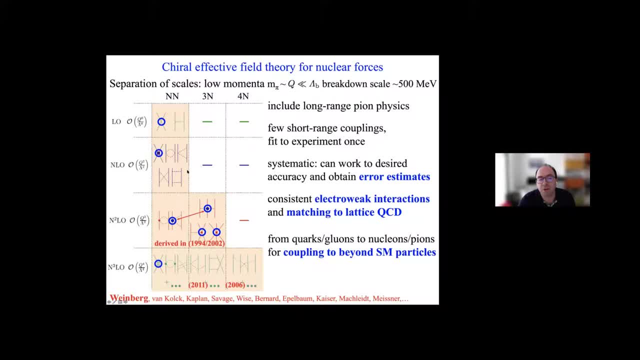 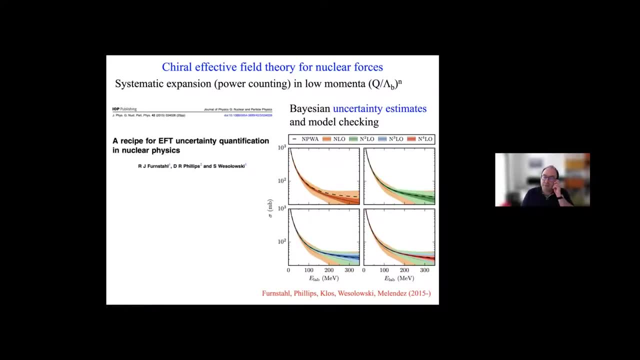 with the external probe, a sub-leading order interaction of the nucleons with the external probe, And there can be also multi-nuclear effects at higher order. Let me draw your attention to some of these. This is something that's very interesting and maybe is also. 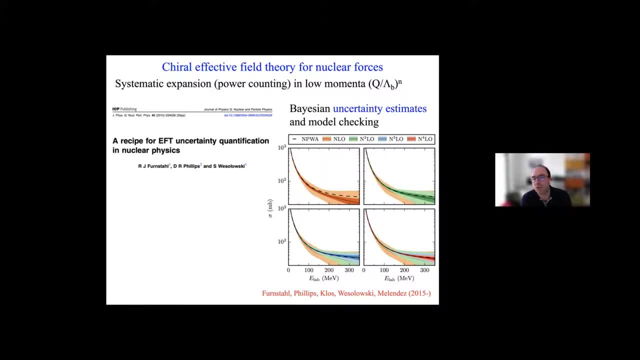 interesting, Could be interesting to you, independent of the dark matter stuff, And it will probably start to play a role also for dark matter nucleus scattering at some point. Namely, there have been a series of papers from about five years ago which combined the systematic 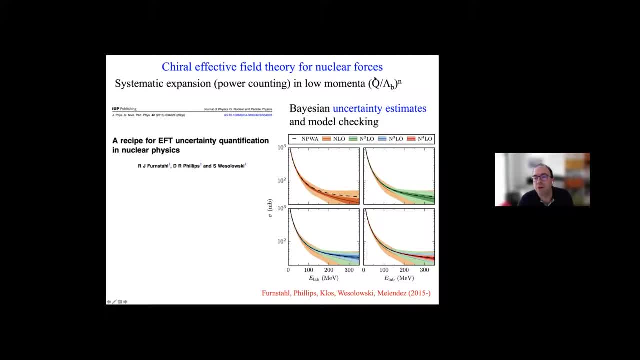 let's say Taylor series type expansion in Q over in momentum and the inter-Q over breakdown scale. So you have this momentum expansion together with a Bayesian statistics to provide statistically meaningful theoretical uncertainties, And this goes under the word of Bayesian uncertainty quantification or Bayesian statistics using EFT. 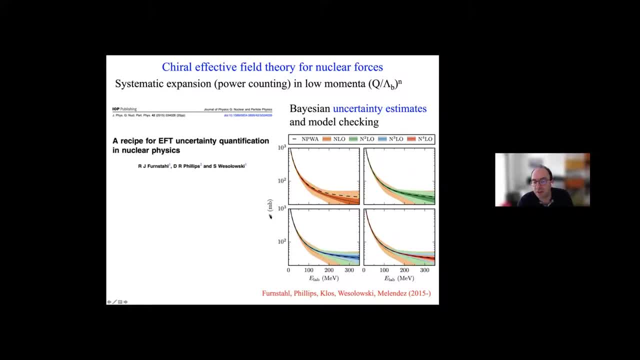 And here you can see, for example, this is not dark matter, nucleus scattering, but this is nucleus And you can see, for example, if you look at this graph, you can see that this is a cross-section for nucleonucleon. 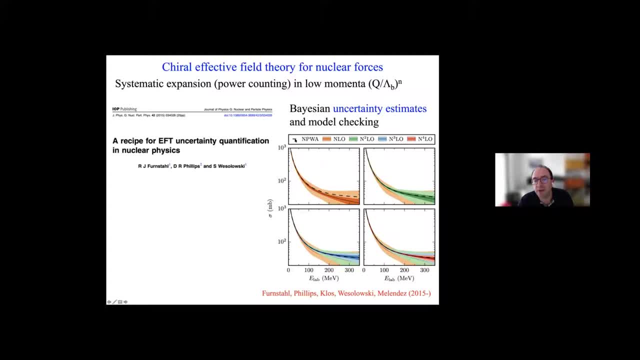 scattering cross-section for nucleonucleon scattering. And here you can see the essentially analysis of the data, which is the black line, the dashed line, black dashed line, And you can see the prediction of the chiral EFT at NLO. 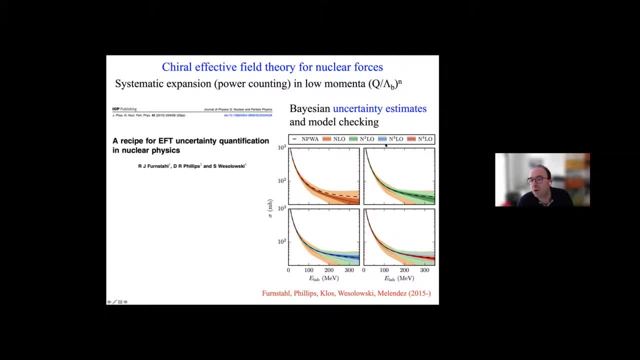 with some 68% and 95% confidence interval using Bayesian statistics, N2LO, green, And you can see from the graph, statistically there are uncertainty bands. So we are in fact in many places in nuclear physics putting theoretical uncertainties because we 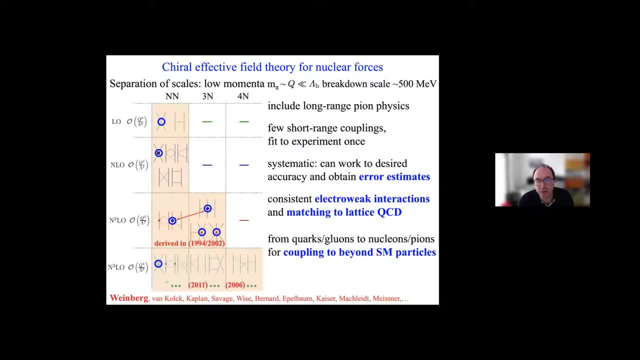 know how the EFT works. OK, so now we're at the level. let me go back where we have discussed the interactions between nucleons and this EFT expansion in terms of momentum, which will be important later. Then let me complete the tour. 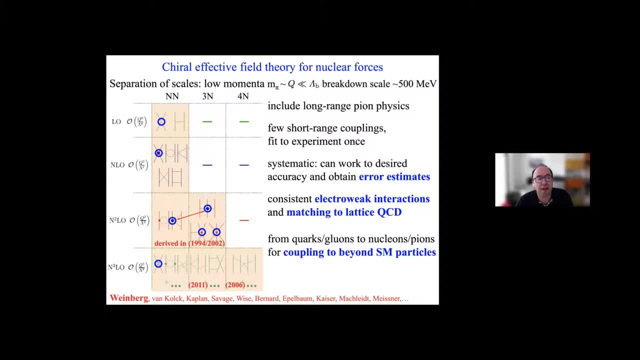 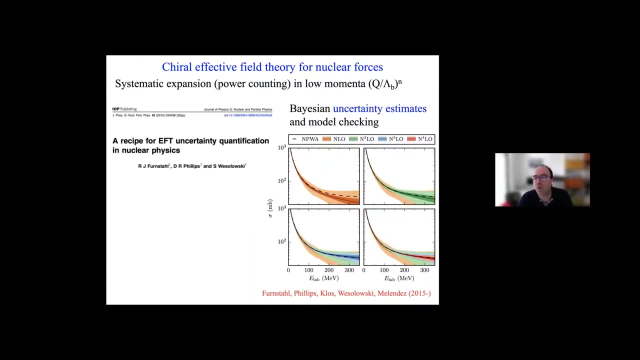 So now we have the uh um, a picture of the interactions inside the nucleus. So nucleons inside the nucleus can interact through short range interactions, through pion exchanges, through three body forces- many different interactions, Um. so how do we describe nuclei then? 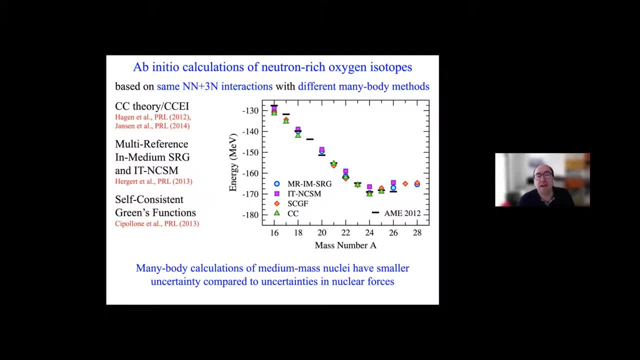 And uh, I will um not discuss this at all. I just want to draw your attention that actually, based on such two and three body interactions, we um, or the nuclear physics community, has developed many different methods- He has just some acronyms for these methods- which provide basically um. 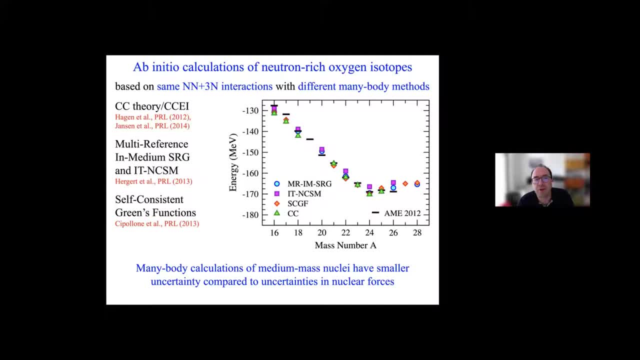 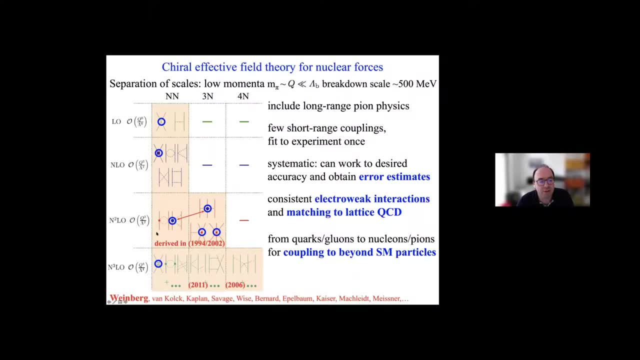 controlled uh solutions of the many body Schrodinger equation, uh based on a given two and three body interactions. So, for example, if you would say I'm going to take interactions up to some order, plug them in. I'm going to plug them into the Schrodinger equation to solve for the ground and 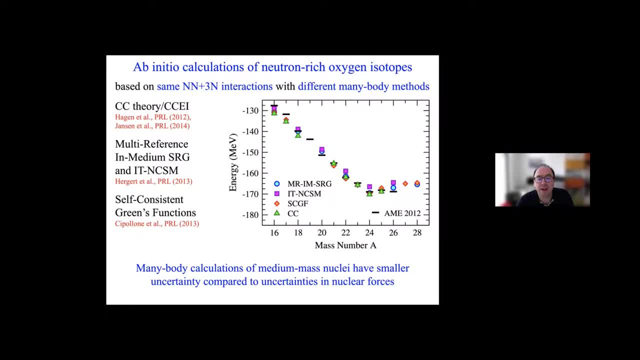 excited states of a given nucleus. Um then this is what you would get for a particular interaction for the chain of ground state energies of the oxygen isotopes- and they are different acronyms here- which also the Schrodinger equation used in the same Hamiltonian but with 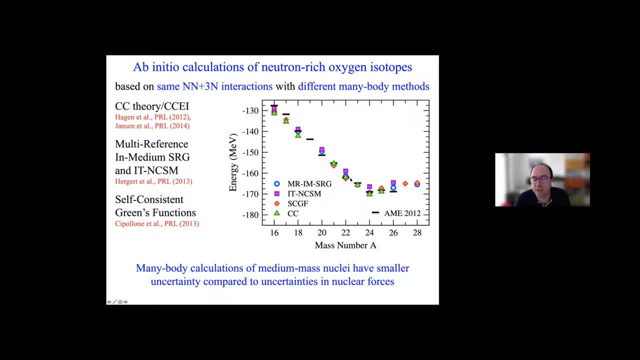 this slightly different: many body truncations, and you can see here from the overlap of the different Colored symbols that the nuclear physicists can basically solve a 20 body problem with a 1% uncertainty for binding energies of strongly attracting nuclei. So this is not yet for you may be too interesting, but it's starting to be interesting because 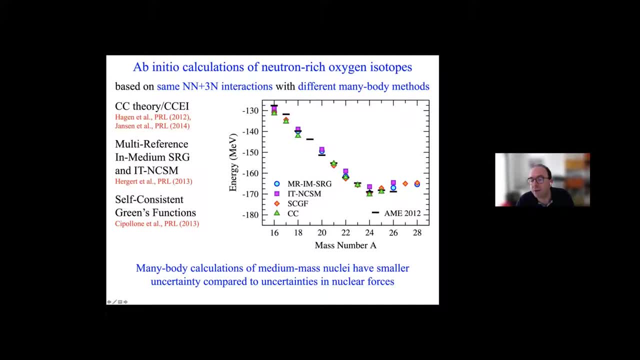 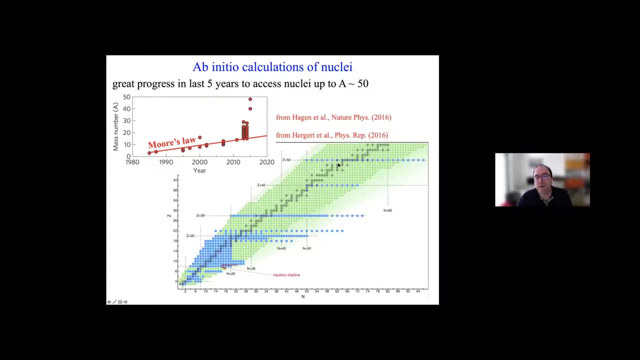 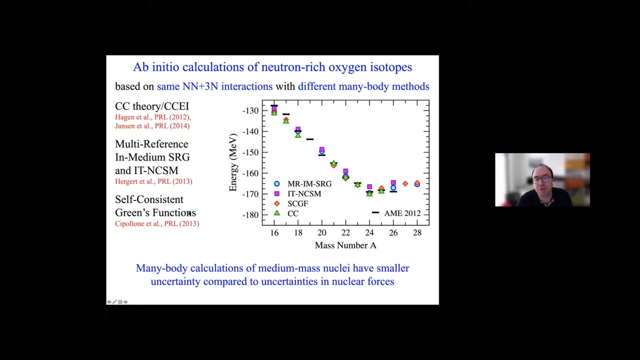 it's. in this lighter region, there are a couple of nuclear targets for dark matter detection which can be addressed with these methods in a what we call up initial way. Okay, Um, and then finally, two more advertisement slides for this. Um, so the real breakthrough of being able to do this, uh, to solve the a body problem. 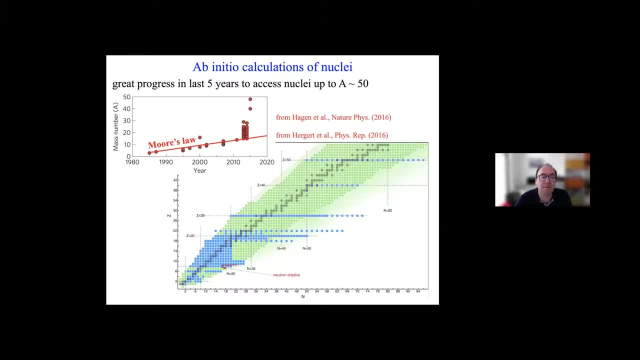 for large a in a controlled way is um, not just computing power. So what we can see here is the heaviest, let's say, the world record in solving an, a body problem in nuclear physics. It went from the alpha particle equal four. 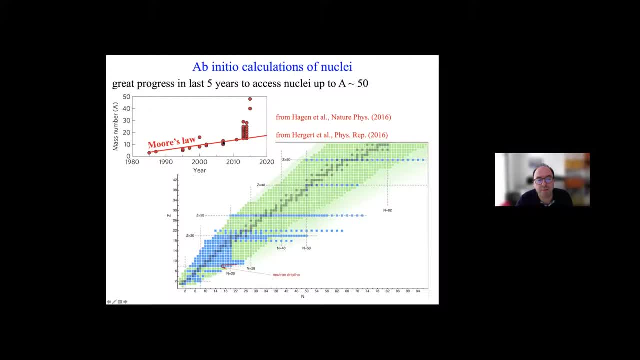 Okay, To the longest time it was carbon 12.. And you can see that if you put all these world records on a line, it's basically linear. The reason for this is that the algorithms used to solve the Schrodinger equation for these points use an exponentially scaling algorithm: exponential in a and since Moore's. 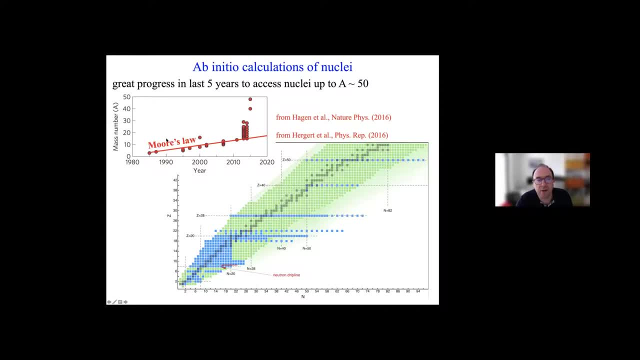 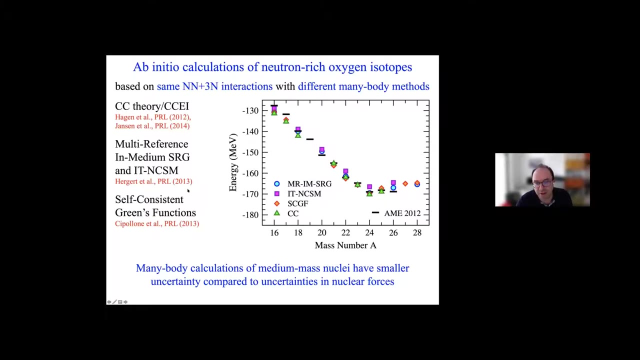 law also improved computer power exponentially. if you have an exponentially improving computer power, Exponential scaling algorithm, you are linearly able to get better in mass number and essentially all of these methods that are quoted here and several others use now polynomial scaling algorithms. 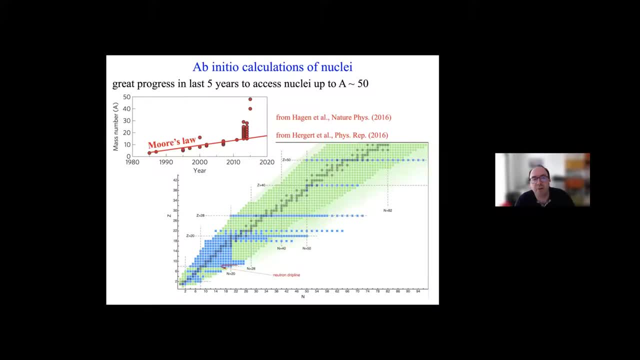 So they more efficiently sample the many body. Hilbert space, And this has enabled a- this is a point from 2016- has enabled the calculation of a nuclei way beyond carbon 12, which you can see from here, Because we are still benefit from Moore's law, but our algorithms scale polynomially. 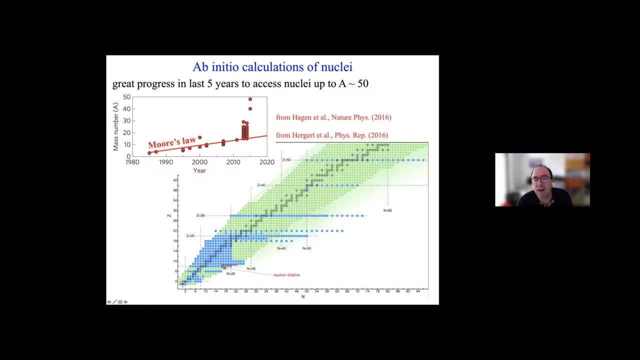 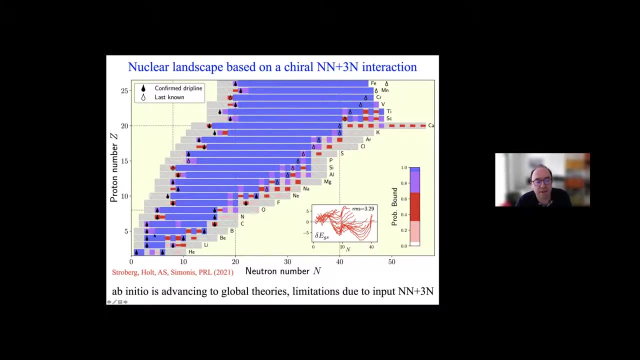 So we are basically able to calculate lots of nuclei and we have calculated in this paper here with Ragnar Storberg and collaborators. We have calculated the 700 lightest nuclei in this way, fully up in the show. Okay, So this is was supposed to be my introduction to 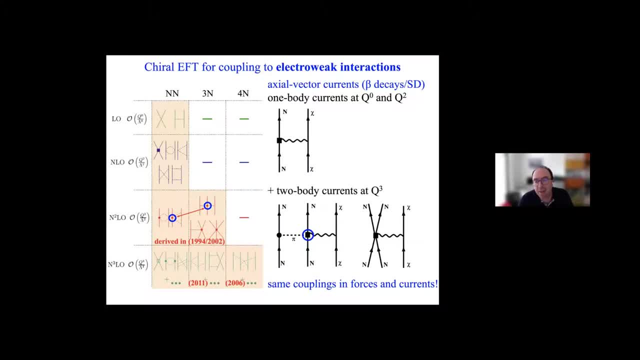 So Strong interactions. And now I would like to tell you one other aspect of strong interactions, coupled to week or later: the dark matter sector, which is important. And then I come back completely to dark matter stuff. Okay, So I already told you, or maybe this is a good point where I can ask: are there questions? 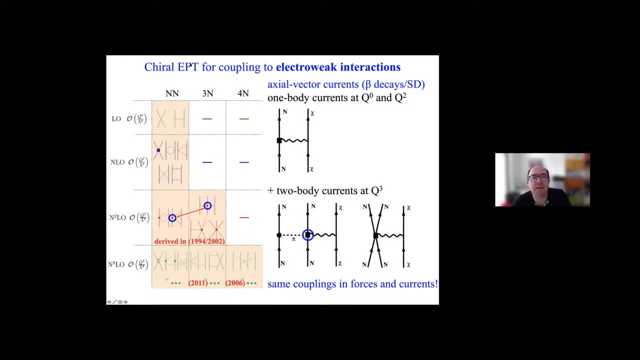 I can see the chats, but I can't see any raised hands or so this you would have to for the failure that you would have to look out for I can see also. okay, So, so, let me okay. So we are now basically at a level of having discussed the interactions between nucleons. 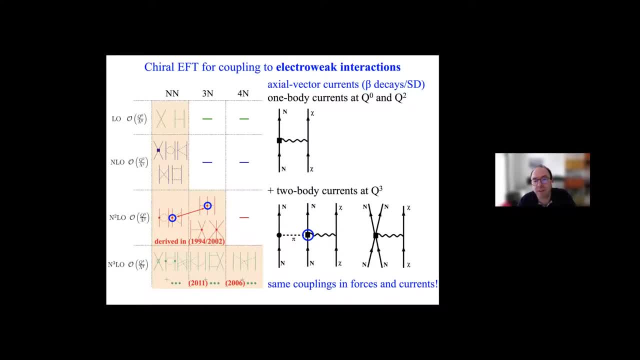 And I've shown you that. Okay. So Nuclear physics has basically triggered by this interest of facilities and astrophysics to understand extreme neutron, which nuclei has developed methods that can solve Basically up to a hundred nucleons or so At some level of accuracy. 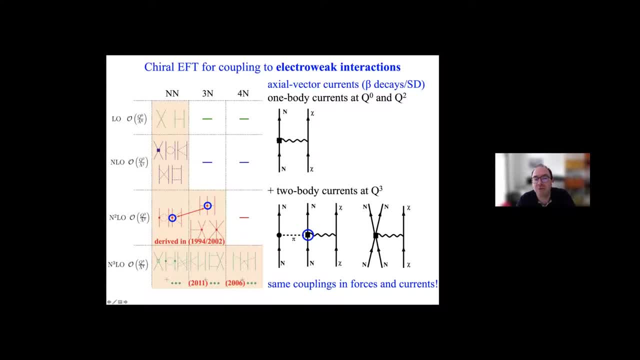 That we can discuss later in the exercises. Now I want to come to what happens if you have a system of nucleons, which is depicted here, and you let it couple to photons, weak bosons or later on to dark matter particles, to wimps- and this picture here is actually a picture for wimps coupling to nucleons, but here i will use 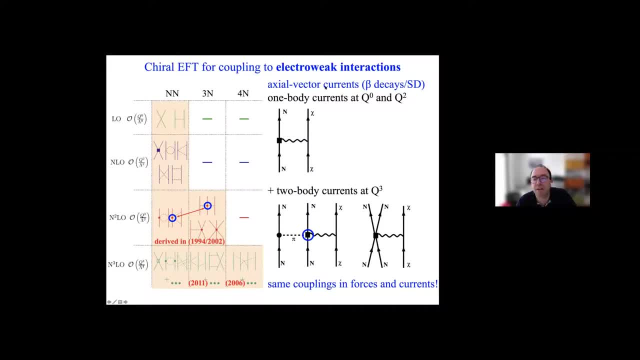 it for axial vector couplings in the, for weak interactions. so, basically, we are doing here beta decades, okay. so, um, if you have a, this is this is a w plus or minus boson, um, and if you have a any external probe that couples to nucleons, i already told you that at the simplest level. 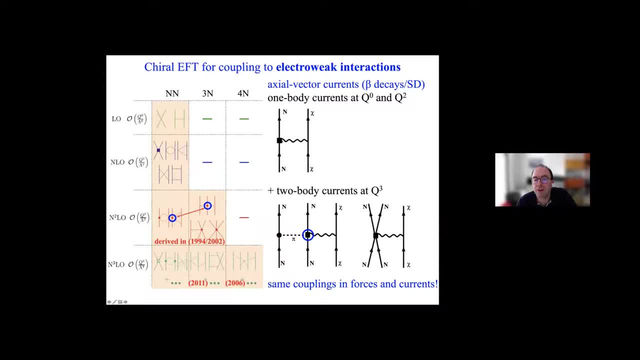 this couples to a single nucleon, and then we call this current current interaction a one body current at the nucleus level- okay, so it's like a one body coupling. or at the weak current, axle vector. weak current couples to an axial vectors, hydronic current. there's a one body current here and in fact, for beta decays. 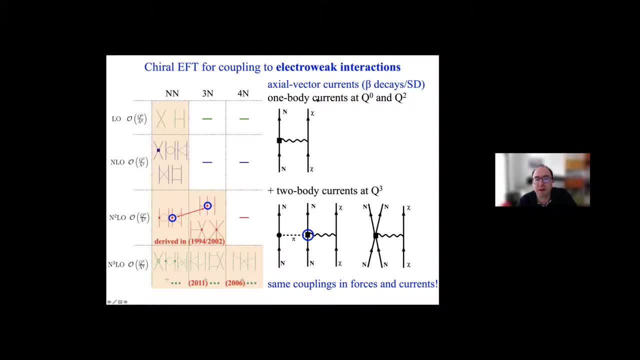 the dominant currents are one body currents, they are. they are at leading order q to the zero, at sub leading order q, squared. but if i go to higher orders, just like we discussed here, for the strong interactions, when i go to the higher order here, in particular for axial vector currents, for beta decays, at the same 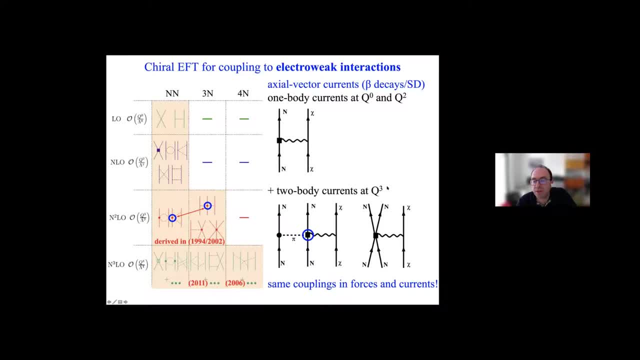 order, as where the three body force is entered, there is are also so-called two body currents, where now i have a, a w plus or minus. that couples not just to a single nucleon, but it couples to a two nucleon system, and this two clone system is not just the product of two one nucleon systems. 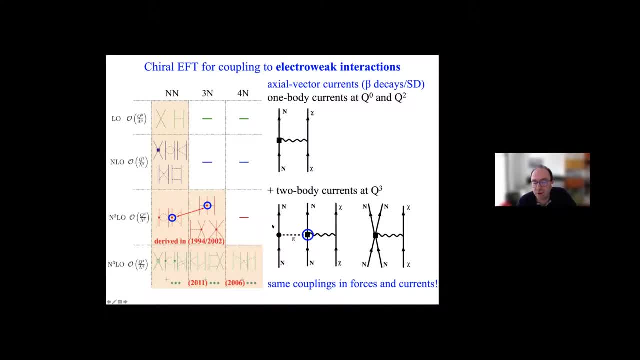 but because of the strong interaction of the two nucleon systems. the two nucleon systems are not interactions. it's so intertwined that it looks like a two body current coupling. okay, and there are two possible two body currents that can enter. one of them is where these two nucleons exchange a. 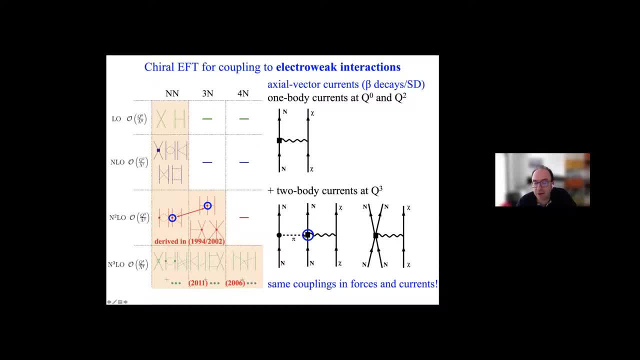 pion and simultaneously to the pion is where the weak boson couples, or the weak cause of boson can couple directly to two nucleons at short distances. okay, and in fact for the beta decay, and this is to some extent also the case for spin dependent. 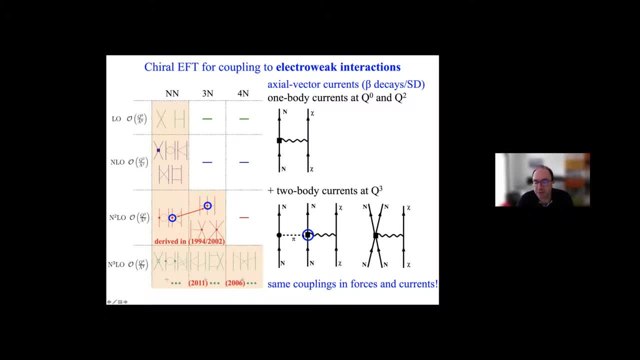 wimp nucleus interactions. these couplings- some of these couplings that are in here- are related to the same couplings as in nuclear forces and it turns out that for beta decays, all two body currents are related to the couplings in the three body force. 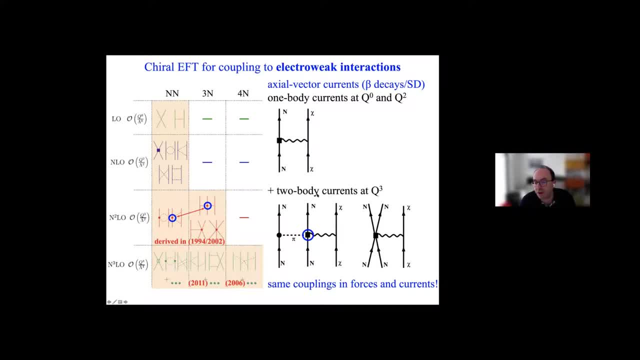 okay, so we can explore these two body currents and see whether they are really there, see whether we actually need this or whether we can forget about it, and i just want to show you two examples that indeed demonstrate that we need it. the first one is from the magnetic sector. 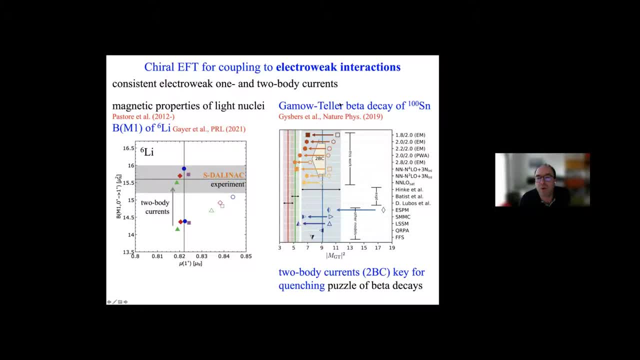 and the second one is from the beta decay sector. these are both recent examples, so what is shown here is a plot of the nuclear for the nucleus: lithium-6, that's an alpha particle plus a neutron and a proton, and lithium-6 in its ground state. 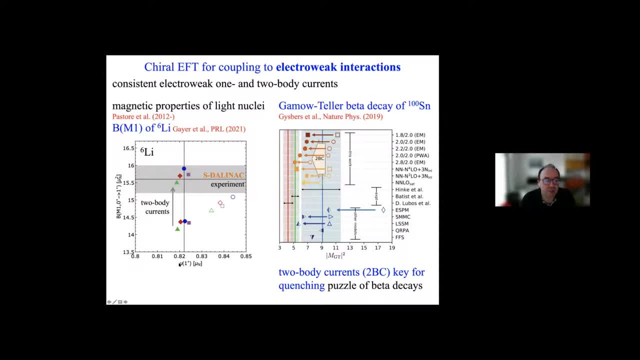 has a magnetic moment. that's the value of the magnetic moment. this is experimentally very precisely known and it also has a magnetic dipole transition strength between the excited and the ground state and this was not experimentally known very well but it was measured very recently. 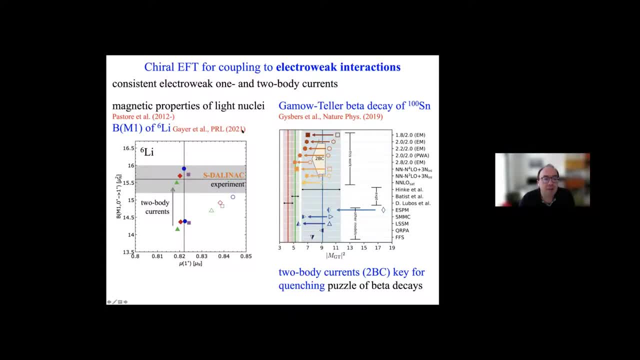 and reported in this pl this year and you can see in calculations which do not include reforms in a magnetic Judy induction current and they look like these bonds are acting as a well-designed coefficient field. at least one times than you know nu to two of these forms of contact will be negative. 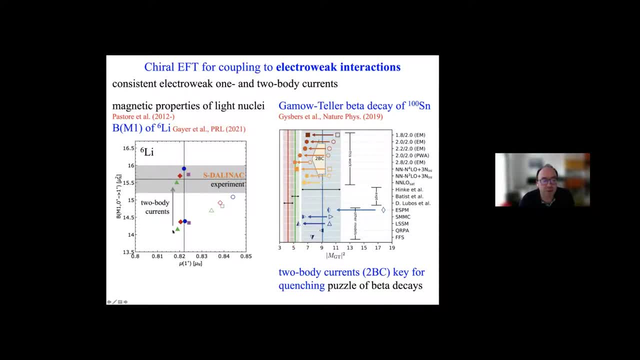 so that is one of the idée we have here: there is to be enough information on these very important there are type of爨 temperature fulfilled Capacities that we are quite curious about: in future not include two body currents, which are the symbols down here, so which mean that the coupling 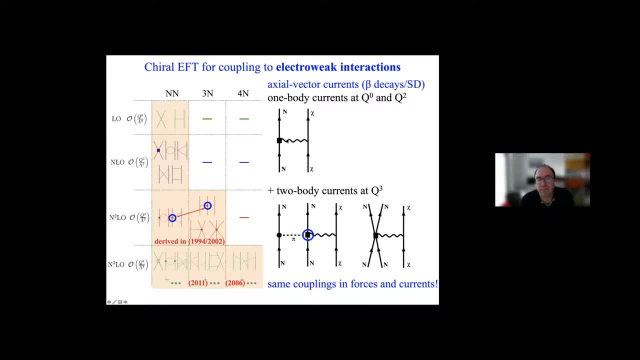 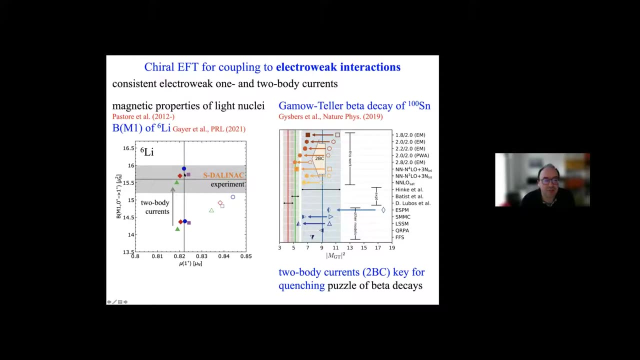 of the photon is just a single nucleon and the magnetic moment is essentially given by the magnetic moment of the individual nucleons. um, that and that gives the proper value of the magnetic moment, but it does not correctly describe these magnetic dipole transitions. okay, and if you? 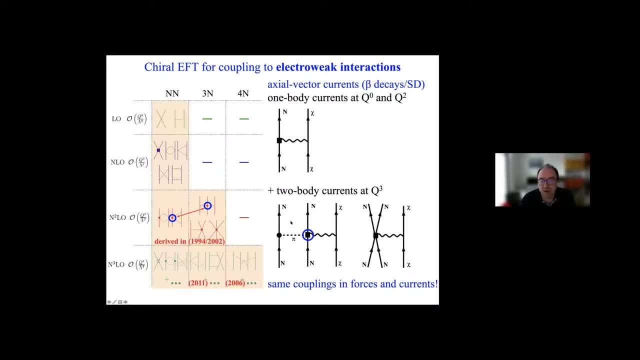 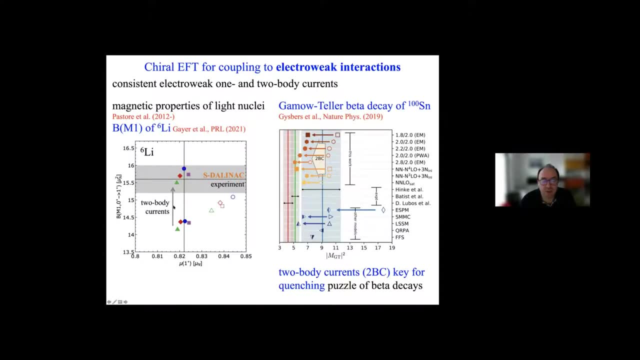 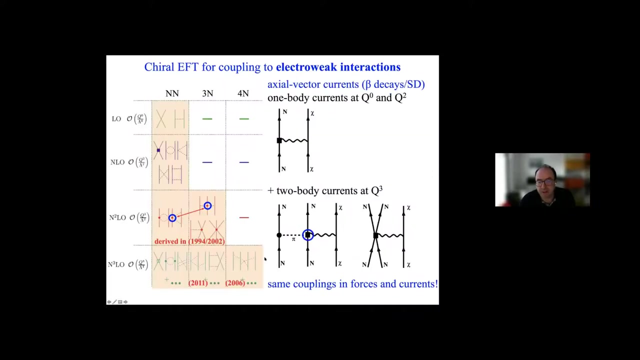 however, if you include the leading- excuse me, the leading predicted- two body currents, then indeed you can without adjusting parameters. the eft predicts you, predicts or post-dicts or agrees with a new experimental measurement. okay, so these two body currents, um these facts that if we have external probes and they couple to a strongly interacting system, 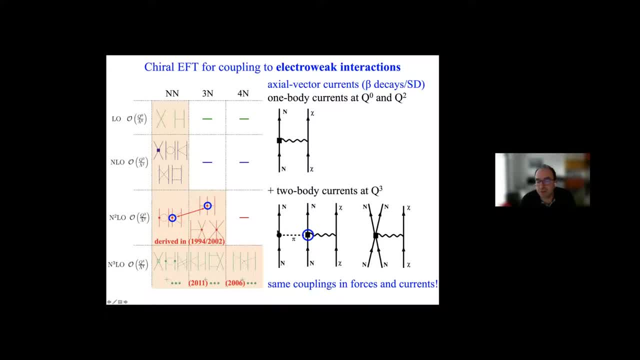 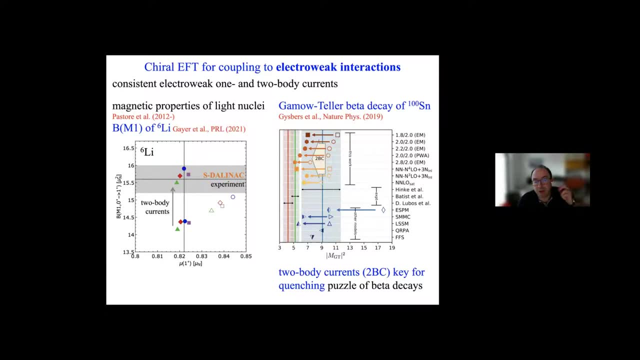 they can couple to a single nucleon or to nucleon pairs. this is an important effect to describe nuclei and their electroweak interactions accurately. this was a magnetic sector. here's a calculation for the gum of teller or for the beta decay of tin. 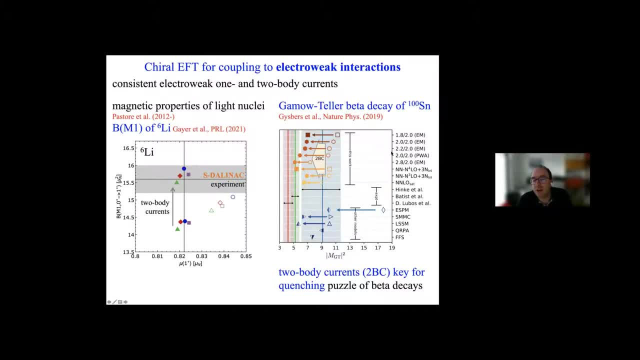 100, a very interesting nucleus, and you can see that there's a range of experimental determinations here, which is um an older one here and two more recent ones over here. so to point to some, what smaller matrix elements for this beta decay this is. the gam says that one is suppose to be four brothers. yes, 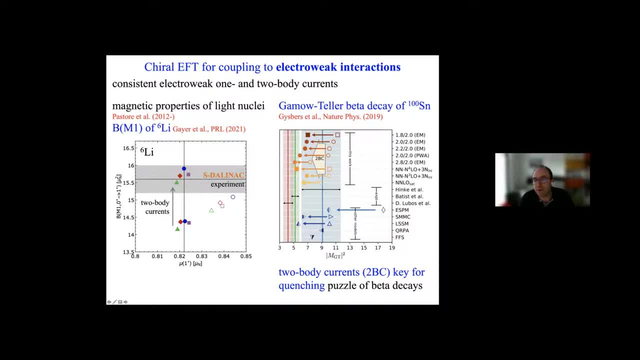 to this beta decay. this is the gum of teller matrix element which is essentially related to the beta decay of team 100, and you can see here calculations using different interactions, knowing no parameters as abinisho calculations. these are inove SAT service conditions arranged up to the minus square even circle. addition Fors Zweig. 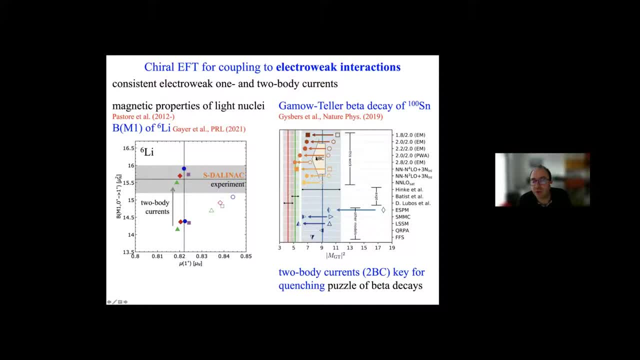 using different interactions and you can see that the inclusion of two body currents is very important and decreases the gamma teller matrix element and decreases this gamma teller decay. and we think actually that these two body currents, here shown by the errors, this quenching effect, is necessary for what's known in nuclear physics as the quenching puzzle to 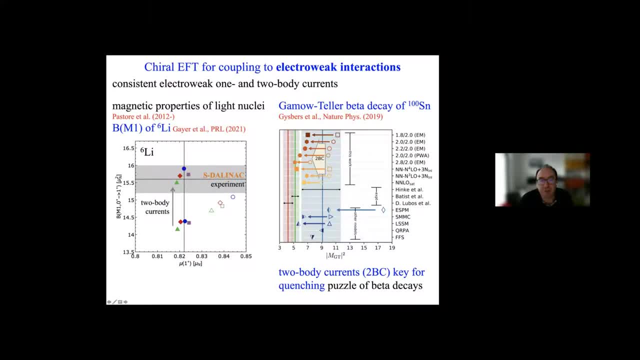 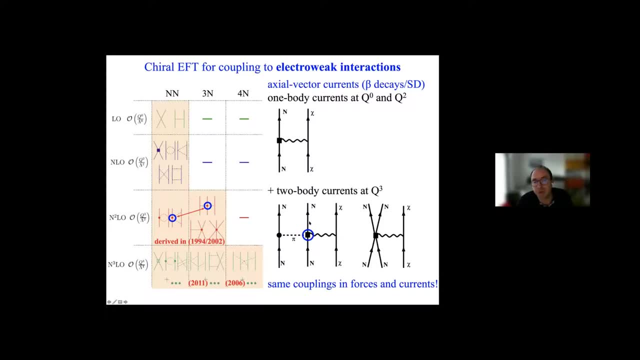 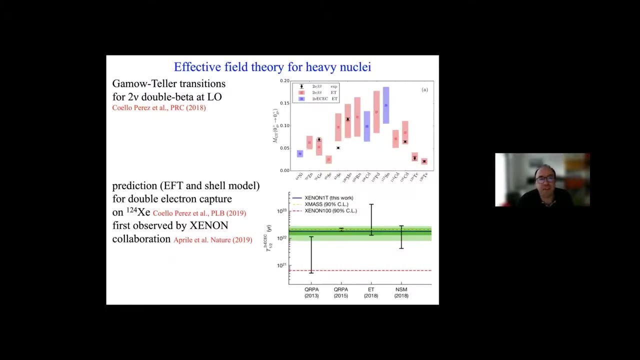 describe beta decay. okay, so all of the physics on this slide: two, three body interactions and one and two body currents are important to describe nuclei and the coupling of nuclei to external probes. i will skip this in the interest of time, but you can ask me about some. 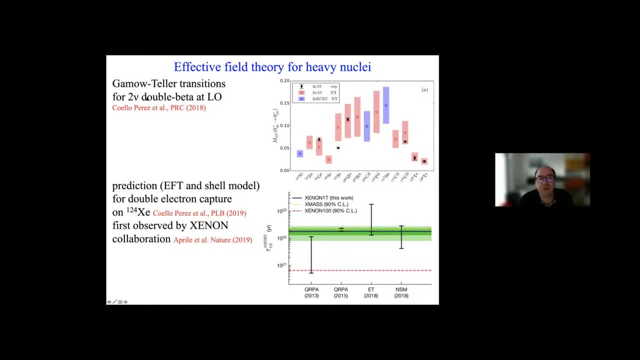 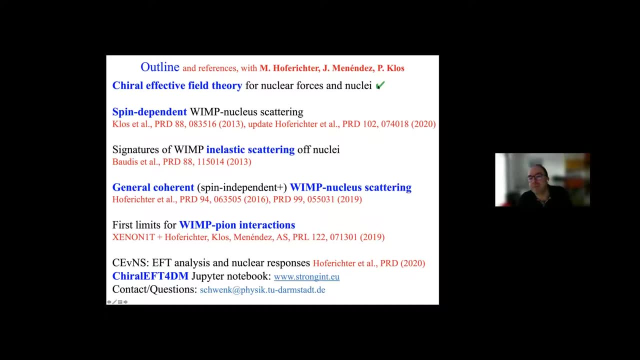 efts for heavier nuclei and which are related to two neutrino double beta decays and two neutrino double electron capture. okay, so now i want to check off the first part for today, the half first half of today. with this, i wanted to show you that nuclear physics has evolved into a field which is very systematic, using effective 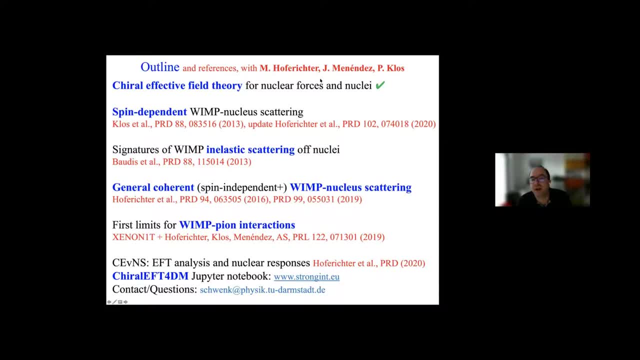 field theories and powerful many body methods to describe nuclei. and this is very important for everything that follows, because if you want to use nuclear physics input, you should always check that what you use is actually capable of describing existing data. okay, so let me go to the dark matter um side. okay, so let me briefly. 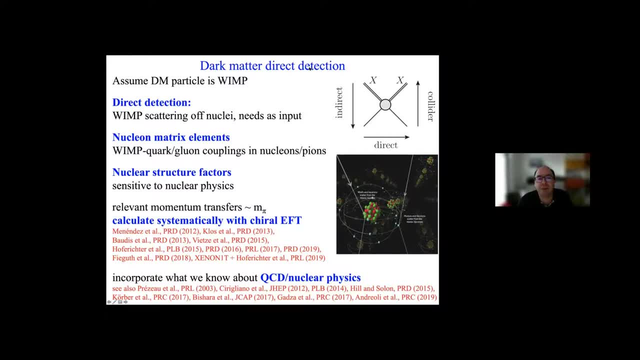 say what i will focus on in the lectures related to dark matter, direct detection. so we will assume the dark matter is particle-like, like a wimp, and then for direct detection experiments you're looking at a wimp scattering off of nuclei. that's where this lecture comes in for nuclear physics and 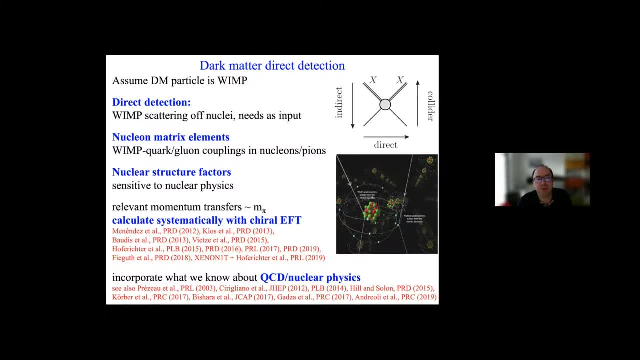 you need as input basically a two point, namely you need to understand how to go from the fundamental level, where the wimp couples to quarks and gluons- bsm level- back beyond standard model level, and then you need to make a transition from these couplings in a systematic way to the matrix elements, where the rims couples to nucleons and 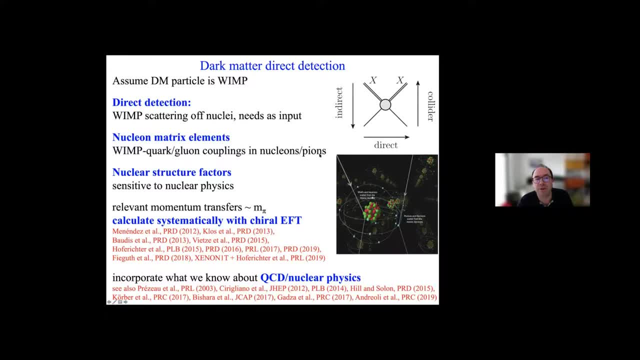 nucleons and pions, which are the relevant degrees of freedom for dark matter. direct detection using nuclei. right, we don't describe nuclei in terms of quarks and gluons, but in terms of nucleons and pions, as i just showed you, and this is goes under the name nucleon matrix, elements or pion matrix. 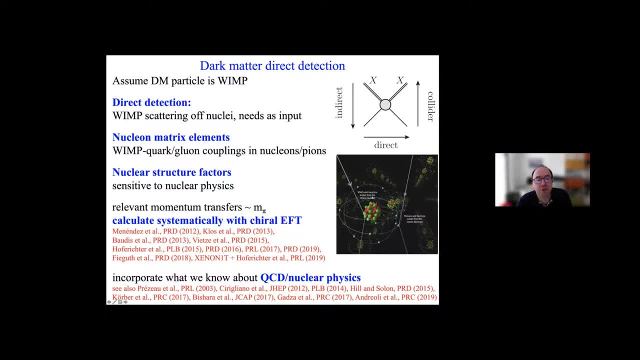 elements, hadronic matrix elements, and then you also need to encode the nuclear structure, physics. how does the nuclear structure, the nuclear chart, emerge? approaches, because a nucleus is not a collection of A nucleons, but it's a strongly interacting system And this is encoded in the nuclear structure. 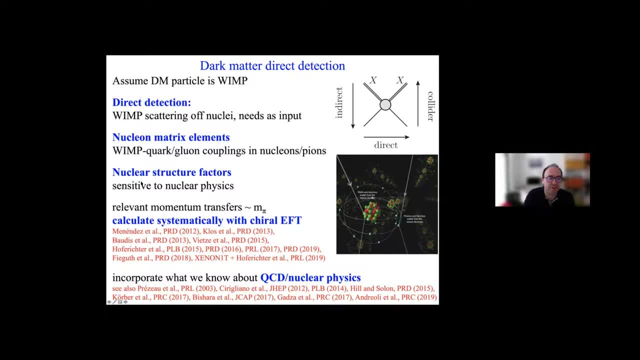 factors or so-called nuclear response function, which is sensitive to nuclear physics. Now, if you look at the direct detection experiments and you analyze the expected recoil from a WIMP scattering off of a nucleus and change it to momentum transfer, then you actually find that the momentum transfer in WIMPs 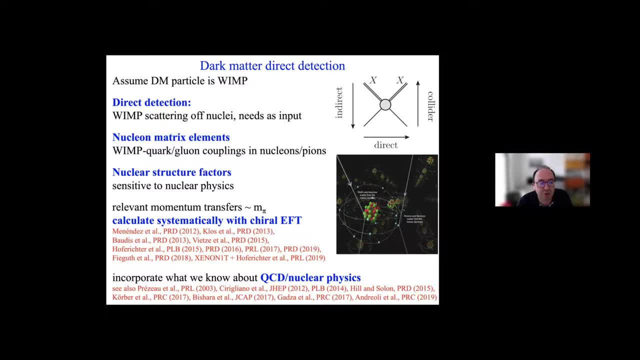 or dark matter particles scattering off of a heavy nucleus, like in this cartoon. here include momenta that are low, so great for EFT, but may reach up to the pion mass, So it's actually perfect for chiral EFT. 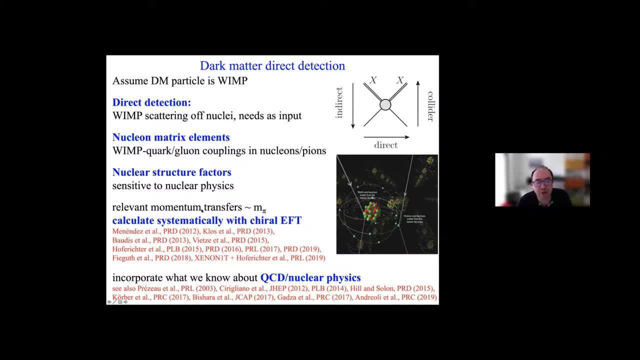 And actually we were triggered to look at this by a colloquium of Laura Baudis in Darmstadt in 2012 and since then have been working on deriving nuclear structure factors and nucleon matrix elements based on chiral effective field theory, to provide input. 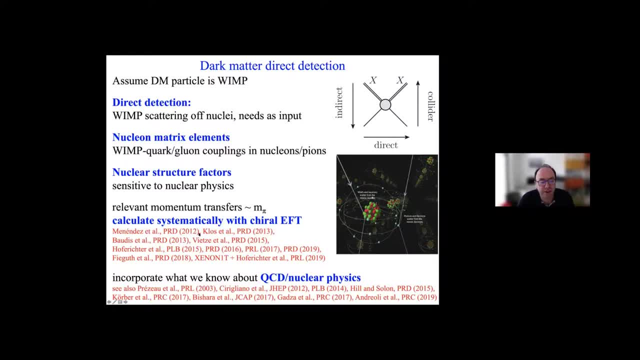 nuclear physics input for dark matter, direct detection. And this is here a series of references. I gave you the key references that we would discuss before And I want to emphasize: there have also been others who, of course, worked on looking at dark matter, nucleus scattering. 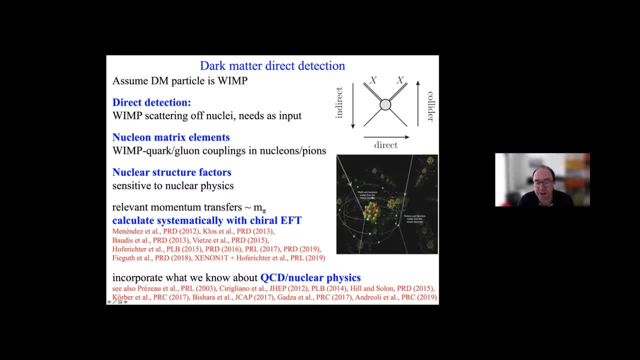 And this is very important- that one includes this correctly, because otherwise, when there is a signal, you don't know what is standard model QCD and what's not standard model physics. OK, so let me put this here, going from WIMP: quarks, carbluon. 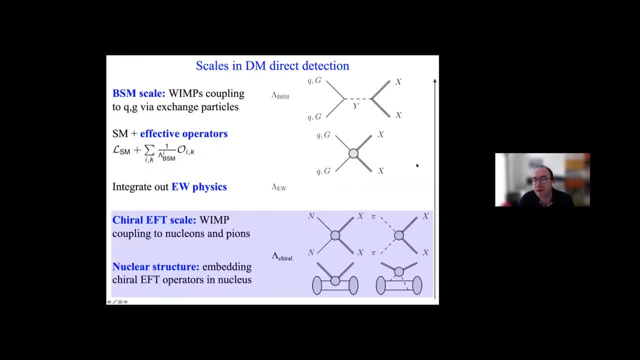 couplings to nucleons and pions on one big energy scale. sorry tower of effective field theory plot. So what I meant before is that we really want to go from the BSM scale where, through some exchange particles, the WIMPs, here the Xs, coupled. 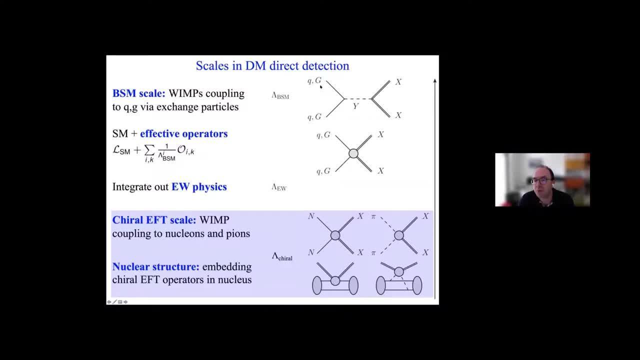 to quarks and gluons. Tomorrow we will actually do this not from that level, but from the effective operator level, where we basically treat the exchange particles here as heavy or we just supplement the standard model by some higher dimensional operators where the WIMPs still 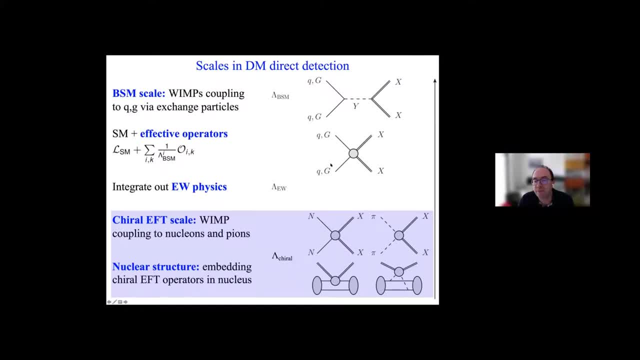 coupled to quark and gluons. Then there are some, let's say running, electroweak, running electroweak physics to be included, to be more accurate. And then we go make this transition not to coupling to quarks and gluons. 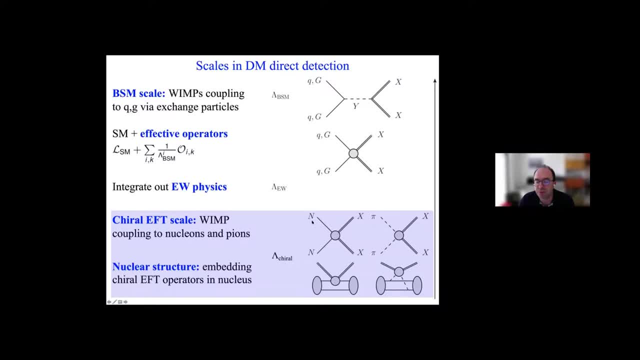 but we want to look at the coupling of WIMPs to nucleons or WIMPs to pions, And this is all the scale of the chiral effective field theory. And finally, if we have understood the chiral effective field theory aspect, then we also 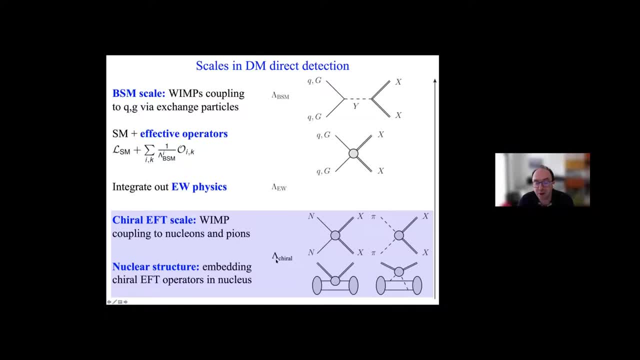 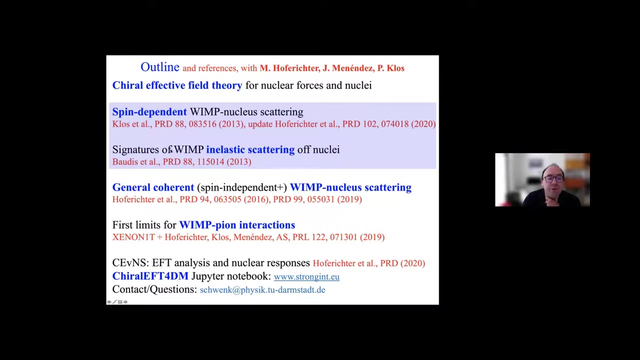 need to calculate the nuclear structure- physics meaning we need to look at the nuclear wave functions and combine this with the EFT operators And with this I would like to start discussing these two topics- for spin-dependent WIMP, nuclear scattering. But maybe this is another point where 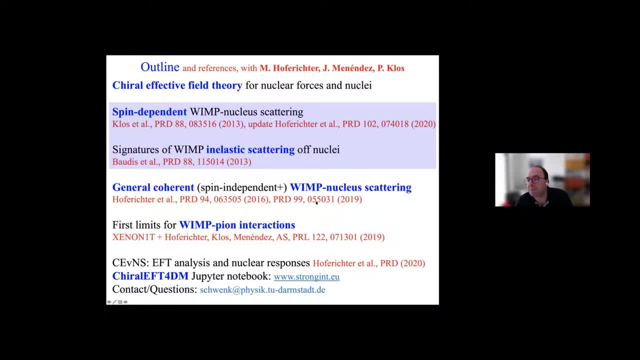 it's good to take a quick break and ask if you have questions. I see there are no questions at the moment. Good, Maybe I can ask the W in EFT field theory approach to make reference to the Nazis of nuclear. And then you discuss the quenching in beta decay. 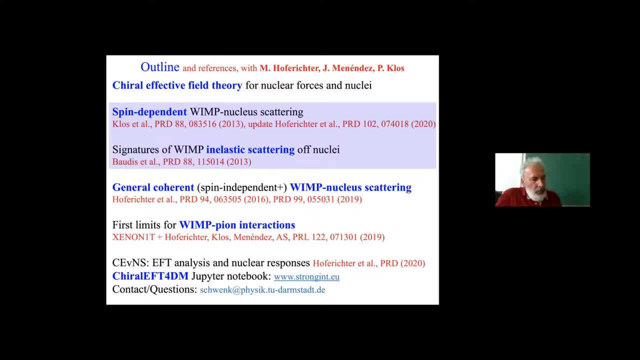 But I need to explain it- with two-body interactions, with two-body currents. So the question is: did you try also to make reference to muon capture? No, not yet. This is what people are working on, So that involves higher momentum. 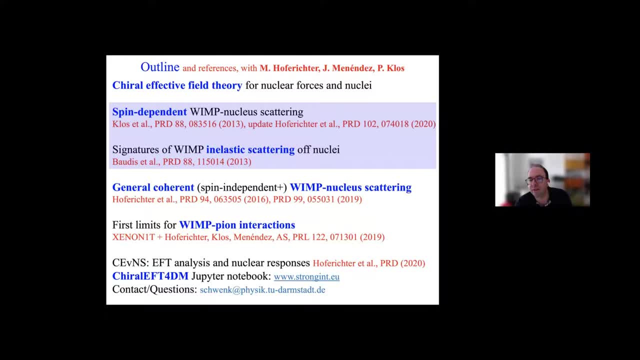 And getting the current, including the current with higher momentum transfer, is a little bit more work. So there are some calculations, I should say, for a few-body systems with muon capture by the PISA group, But for nuclei there are no calculations yet. 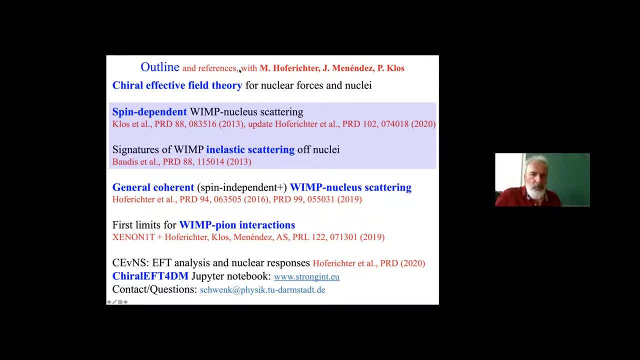 People are working on this. OK, Let me actually, before I go here, maybe I'm going to do a short question, So maybe there is some questions. Somebody is asking whether the mass of the mediator should be different from the mass of the pion. 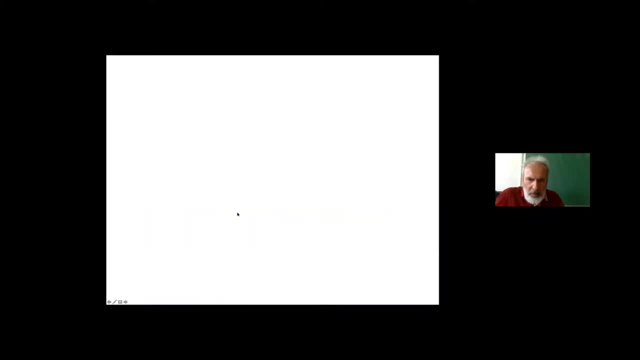 In the effective approach. I think in chat do you always assume that the mass of the mediator is of the order of the mass of the pion. No, we don't assume that. In fact, this is like We have the BSM scale here. 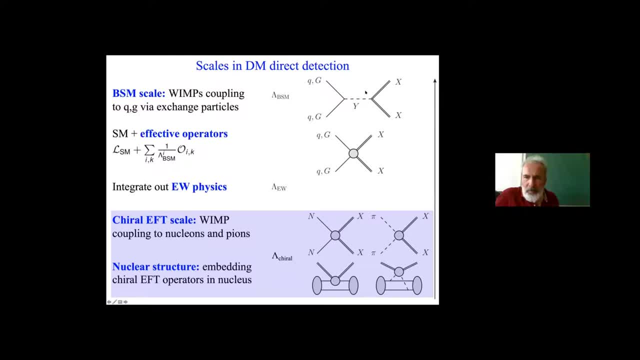 So at this even heavier scale, And we will represent this part here through basically higher dimension operators to the standard model, So where the exchange part is treated as heavy, much, much heavier than the pion, And for us it's repulsing inter or some other ways. 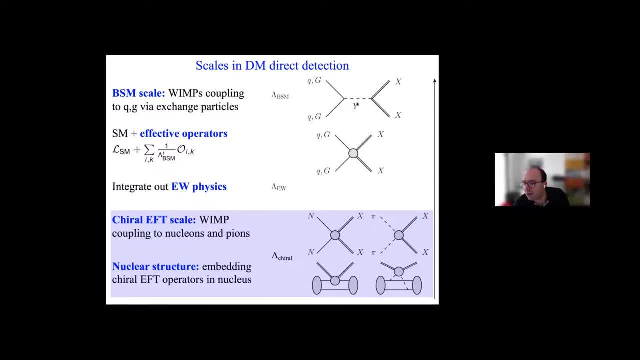 OK, Thank you. I think your question was about why, here for the heavy people, Yes, OK, For us, the mediators, at this level, here, of course. then there are pions, So yeah, So this is not, these are not pions. 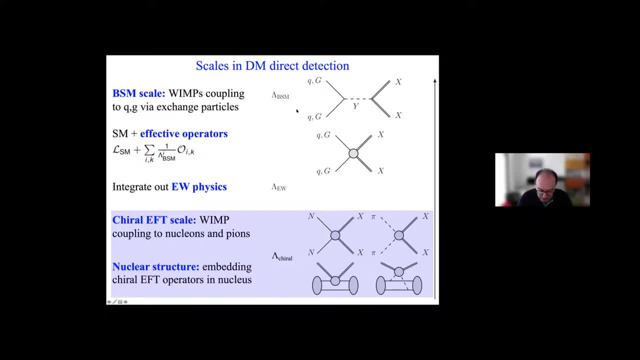 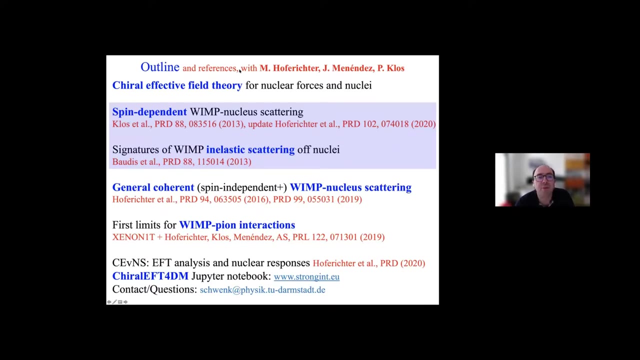 Maybe just so that we're all on the same scale with nuclear physics and WIMPs. I thought I could draw a couple of simple pictures here on the iPad first, before we go OK On to discuss spin dependent with nuclear scattering. I'm not sure how we'll be doing time wise. 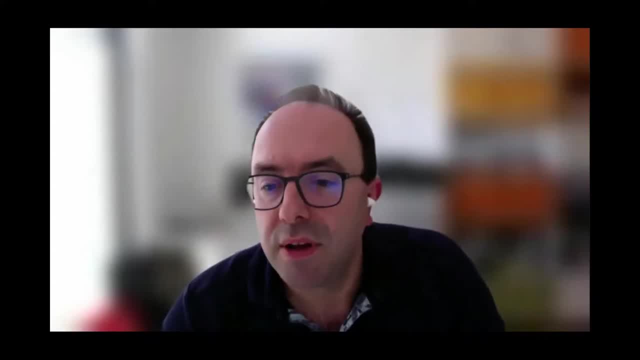 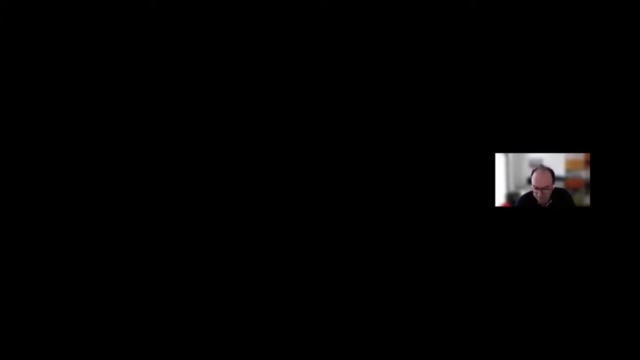 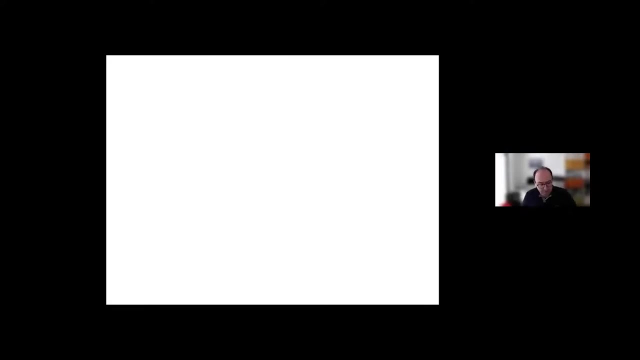 but I still want to try this, So let me share here. switch to the iPad. OK, So let's talk a little bit more about WIMPs. So let's talk a little bit more about WIMPs Coupling to nucleons. 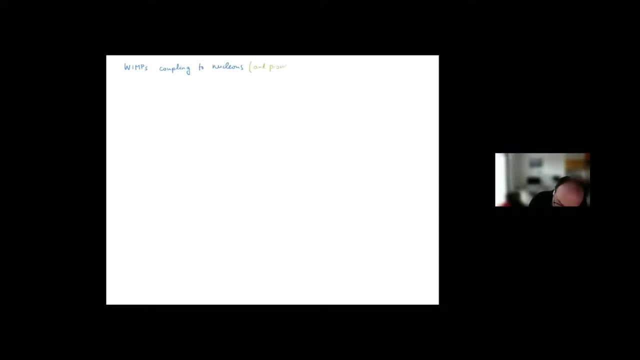 Put in brackets and pions. but I will just comment on this in a second. OK, So since nucleons are, we distinguish some couplings there, and since nucleons are non-relativistic, they are all bundled. There are many, They have. 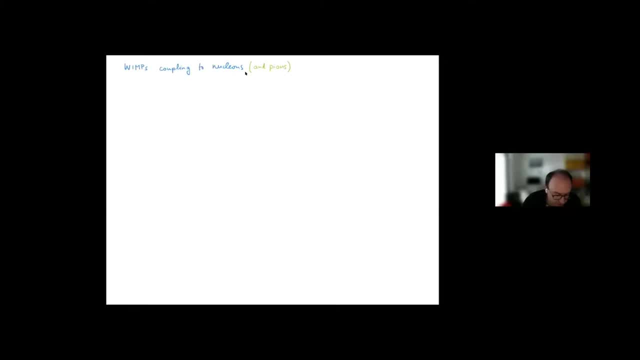 OK, A spin. They have a momentum. So there are many possible things we could couple to for the WIMPs, to the nucleons, And in fact you probably know we distinguish a coupling to an operator. that's basically the identity one. 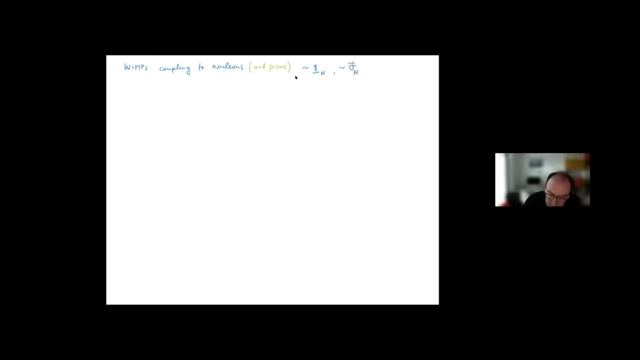 Or we could couple to the spin of the nucleon- So the spin of n is supposed to be neutral- or proton, Or we could couple to something that is momentum suppressed. We put q to something, We put q to some power times 1 or spin. 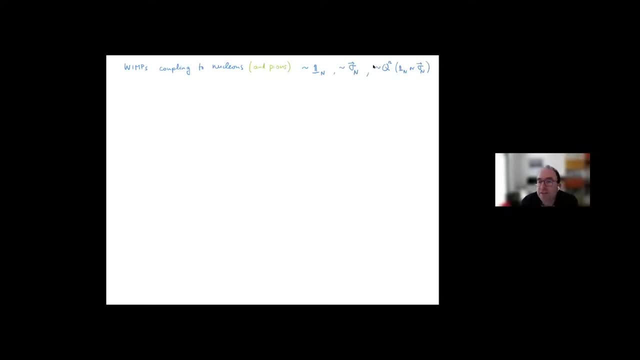 OK, And I will not discuss these today at all. These are momentum suppressed interactions, OK, And in fact they are much weaker than these two, although there are a couple of interesting responses here. Now this is coupling to nucleons. 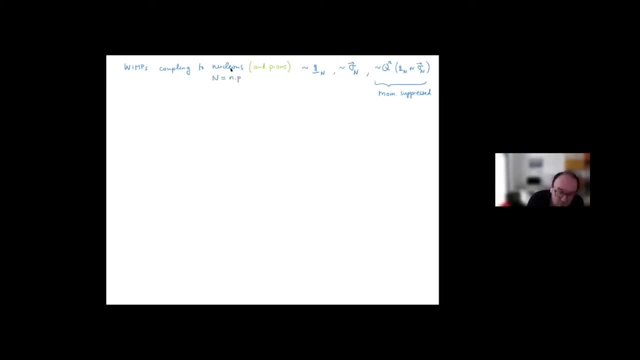 So a single n neutral or proton, But for us these are bound inside a nucleus. OK, I hope you've got an idea of what I'm talking about. Thanks, Thank you, Thank you, Thanks, Thanks, Thanks, Thanks. 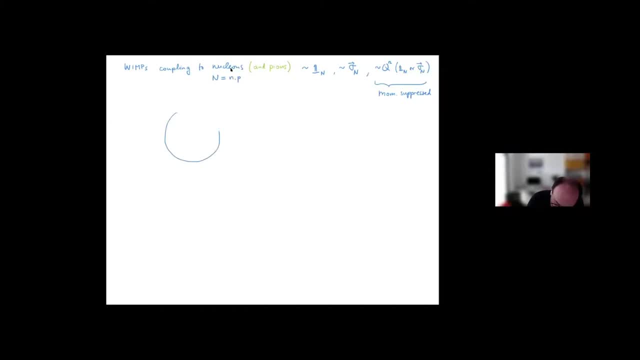 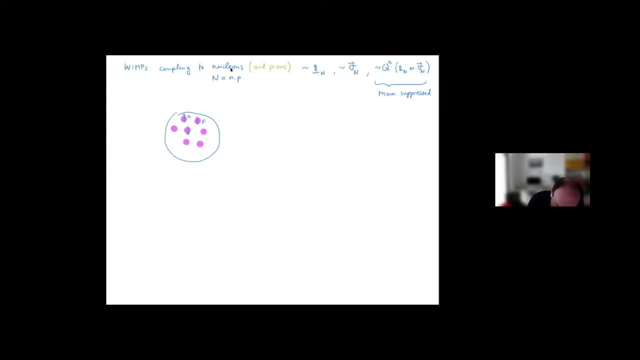 they have spin up and down, And sometimes in a nucleus there's an odd number of nucleons, there's a single. So now if you have a coupling that's of this type here, that couples to the nucleon without knowledge of its spin or its momentum, so then this coupling you can basically in 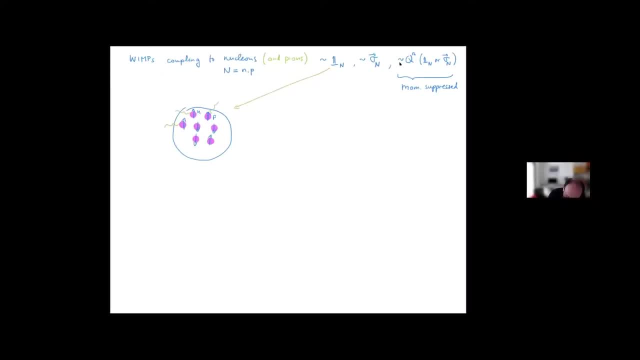 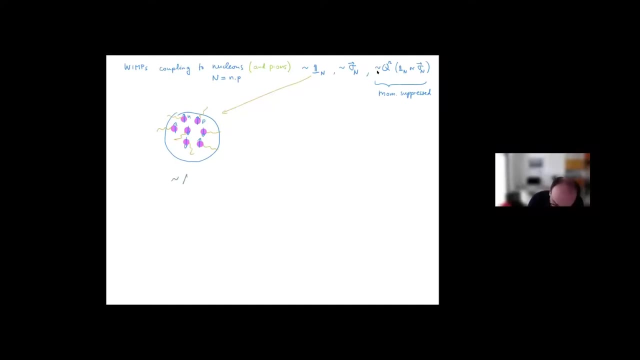 this picture here, couple to every nucleus nucleon inside the nucleus And in fact this response goes as the number of nucleons A, and we call it a coherent response. And one type of coherent response is the spin-independent response, Si. 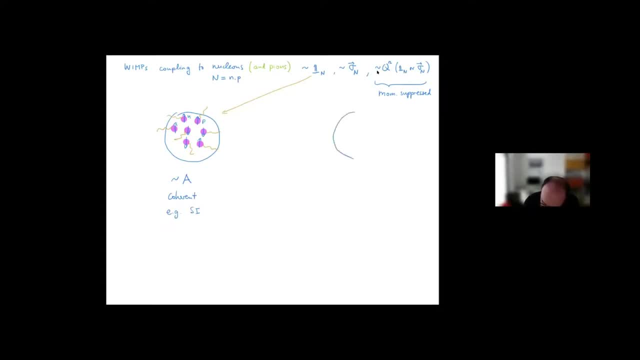 Now, because I am So, because of the interactions inside the nucleus, these spins always pair together inside a nucleus to form a spin-zero pair. let's say j equals zero. The picture is a bit more complicated, but for our simple picture here, iPad picture. 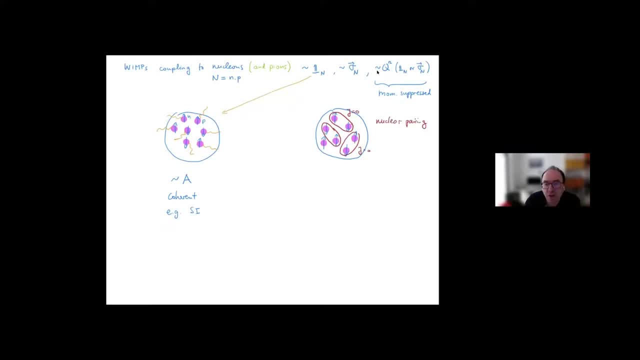 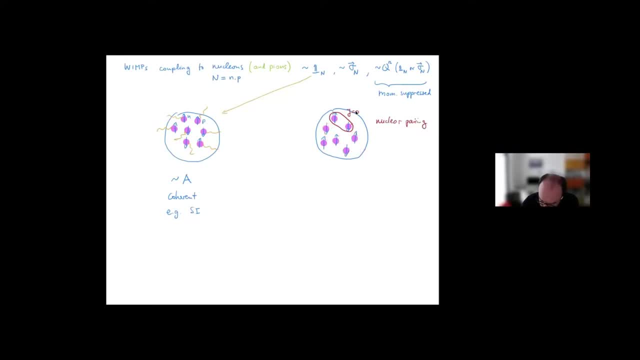 Sorry, let me then, so that you're not confused with: j actually call it s, But because this pair has no spin, the response from this and this nucleon cancels And in the end for a spin-dependent coupling, it's a spin-independent coupling. 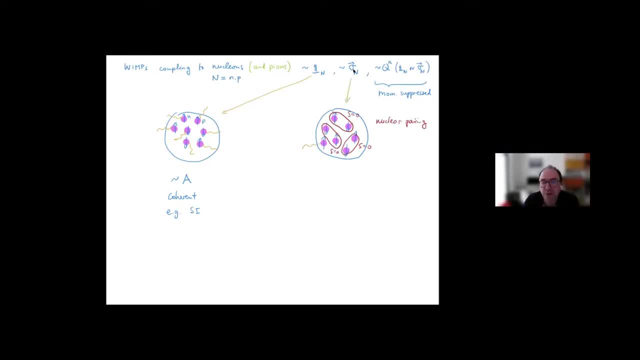 We only couple at this simple picture to a single nucleon. So this response here is this coupling. This response of the nucleus is not coherent, but a single particle And you get an order-one type interaction. Of course you know this from the spin-dependent interaction which we want to discuss. 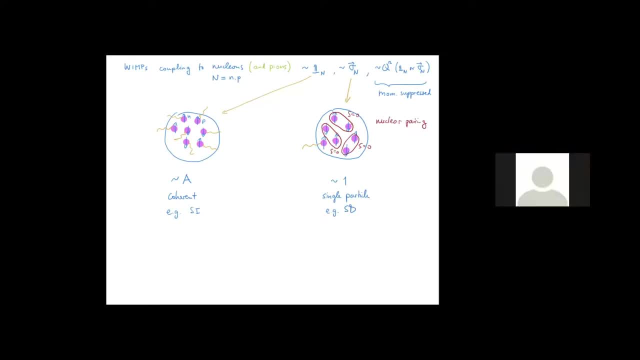 There's a question from Gora. Yeah, Sorry, I'm a little confused here when you say coherent, because even for a spin-dependent also, you are summing over all the nucleons. So you are doing something similar that you are doing for a spin-independent. 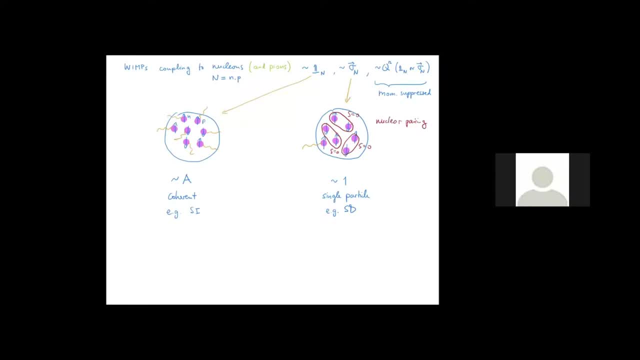 Then why it is not coherent. It is coherent, but it is canceling out, isn't it? Yeah, with coherent, we mean that they all add together, And in this case they all add in pairs to zero, and there's only one response left. 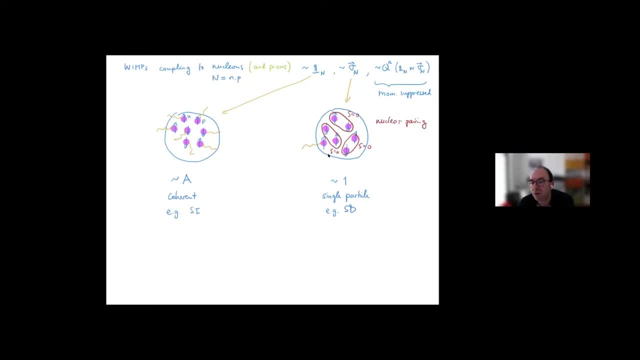 So the response of the entire nucleus. It has a similar cross-section as if you're scaling off a single nucleon. They still couple to everything, but it incoherently adds together: Okay, Okay, But still we are adding them. 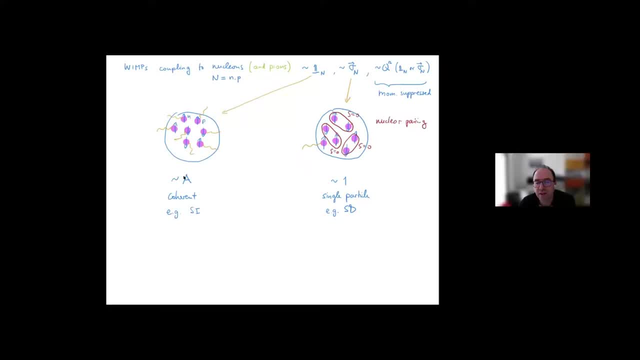 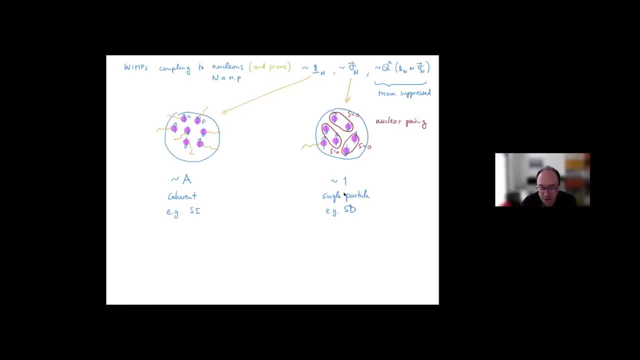 have a much larger cross-section than the single particle response. So let me put some figures here. And it's also clear that anything momentum-suppressed- unless you have very large momentum transfers- any momentum-suppressed will be much smaller. Okay, So basically, to organize your momentum-suppressed is really weak. 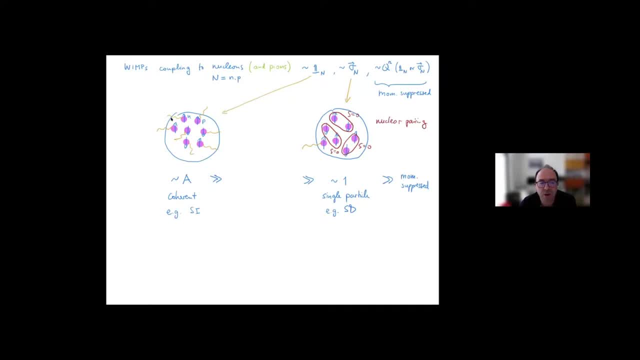 Single particle is next largest and coherent is the. You get all the power of the nucleus because it scales with the number of nucleons. We don't get to this today, but at the end of tomorrow. I will tell you that in between here, if you have. 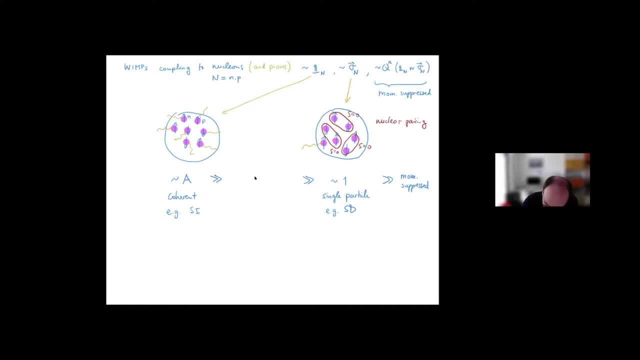 Okay, Okay, Okay. If you have these nucleons exchanging pions here- Oh there, We have a race down. If you have a coupling of WIMPs to pions, This gives you a response which is somewhere in between scaling with A and scaling single. 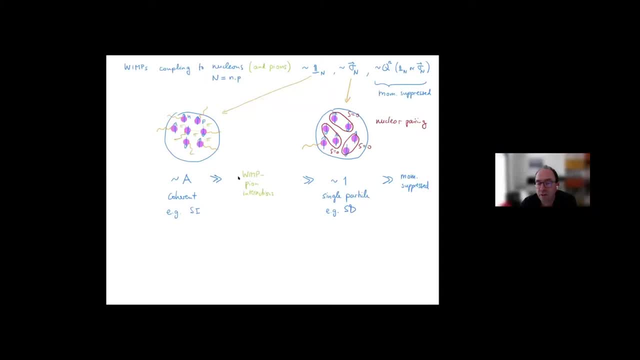 particle-like, Okay. fraction of the number of nucleons. it's a question from, yeah. so on the right side you draw a picture of an odd mass nucleus, illustrative illustration. and if you have an odd, odd nucleus, do the responses add up? so if you have an odd neutron and proton, 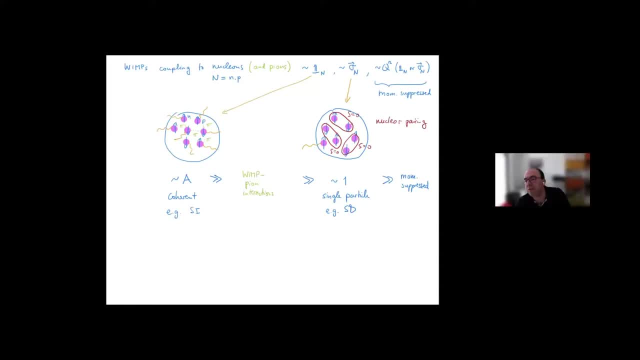 then you will still pair the neutron and proton together for most nuclei, okay, um, and so then it starts to depend on the nuclear structure. okay, thank you, yes, and it it depends also on. then we have to distinguish. that's a very good question, katharina. then we have to distinguish between the coupling to the rims to the neutron. 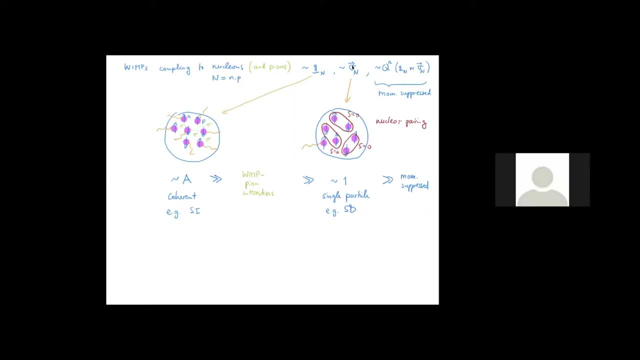 or the proton. okay, thank you. okay, so this is sort of our big picture for the, the lecture that we We will start here at the single particle-like cross-sections And tomorrow we do everything that's coherent, because for this we need some more. 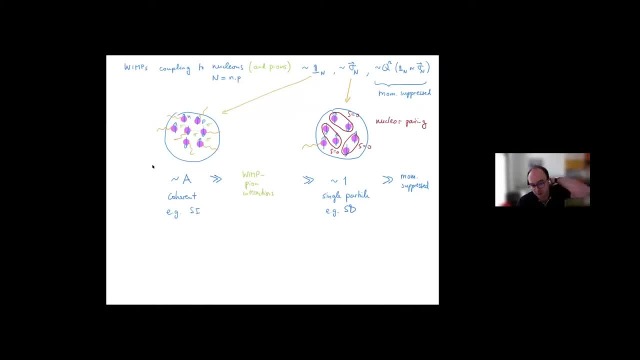 I want to do some more iPad framework and give you some details, But for this, just remember that there is this interesting WIMP-Pion channel and it's actually more important than spin-dependent WIMP Nucleon. So with this, I will leave this and come back. 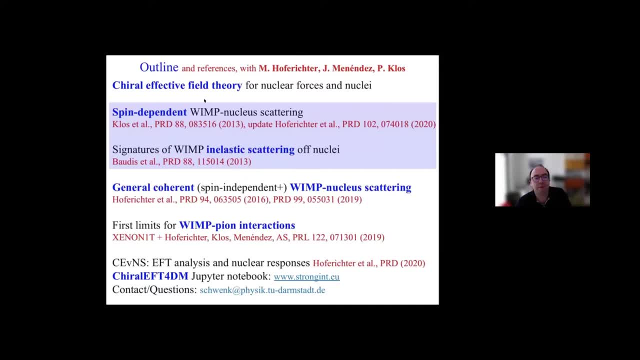 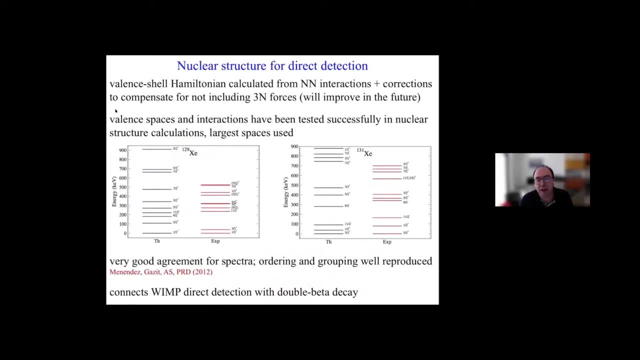 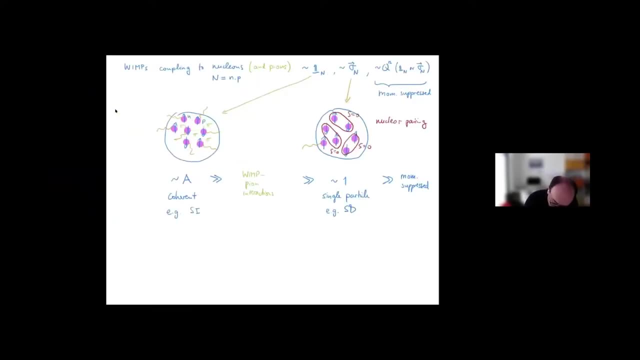 to here, namely, we start with spin-dependent WIMP Nucleon scattering. So now, what's important to me is that unfortunately for the calculations, I could also maybe do this here. So for scattering, this is proportional to the final nucleus. 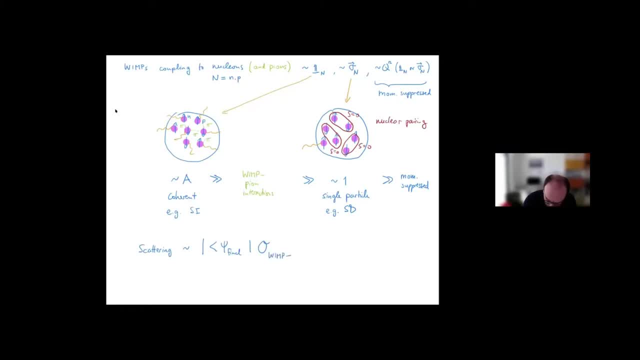 The operator that describes the coupling of the WIMP to the Nucleon or to Pion or to whatnot, psi initial. And so this here we have derived, based on Chiron EFT, But for xenon, and most of my examples will be for xenon. 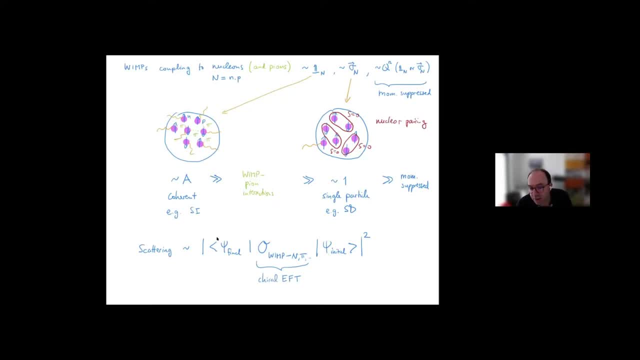 we can't calculate the initial and final state based on Chiron EFT yet, But here for these we use Basically the nuclear shell model. Probably on a time scale of the next few years we will have a good handle of xenon as well in Chiron EFT. 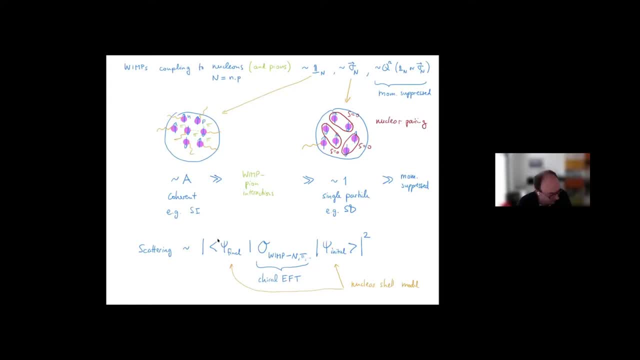 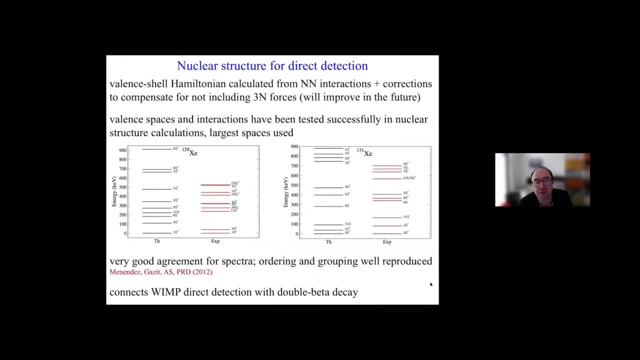 And then one can do the combined thing in Chiron EFT and do order by order estimates as well. OK, OK. So now I just want to show you that for the shell model actually it can predict very well the structure of xenon nuclei. 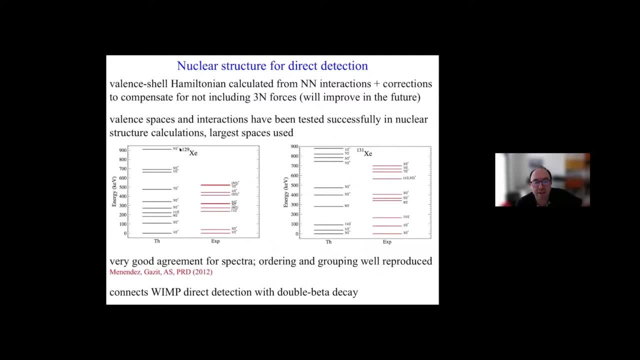 So these are the two hardest nuclei, the odd mass, xenon 129 and xenon 131.. This is calculated based on a Hamiltonian which is built from two body interactions, And then there are some corrections to compensate for things that can't be included yet. 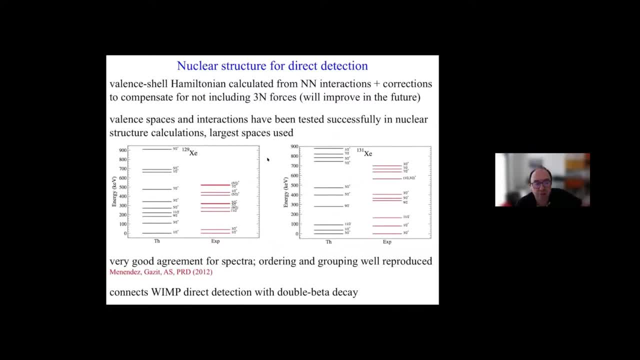 It has based on a very large diagonalization And this Pretty good agreement for the theoretical spectrum compared to experiment. The lowest two states here are in the right ordering. Then there's the next four states are also here. Also, you can see here that this triplets of states is there. 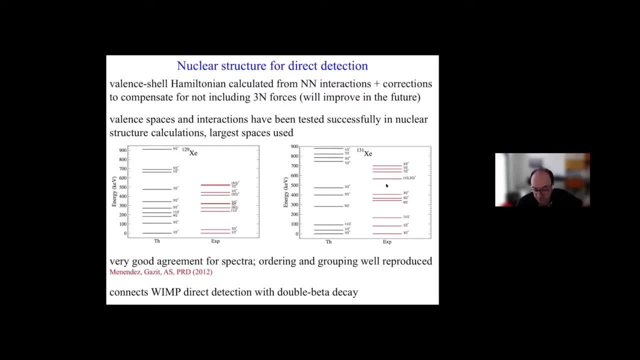 The next triplet is there And the next four states, So this looks pretty good. Actually, I want to encourage you that if you use nuclear physics for dark matter, diode detection, ask the people who provide it for nuclear structure input, because here 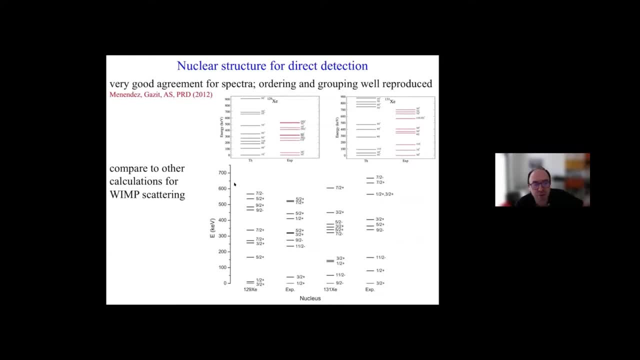 there is a figure from a paper which I will not reference just to not put anybody on the spot, But this is also what is considered a good nuclear calculation and provides some rates for nuclear scattering the same xenon nucleus. This is the calculated spectrum from ground state up. 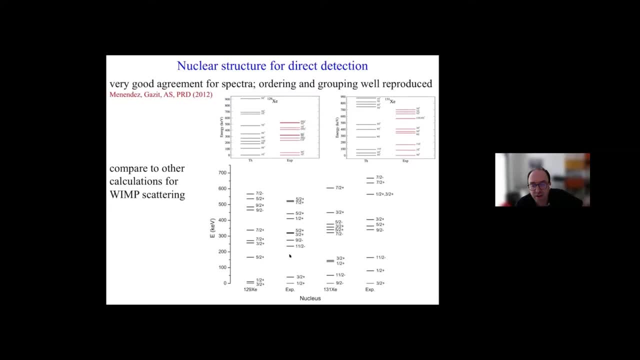 compared to experiment And you can see here that the 11.5 minus state here, the next state, isn't even in the spectrum for the 131 xenon nucleus. The lowest states are not even the ground states. So there are some non-trivial checks. 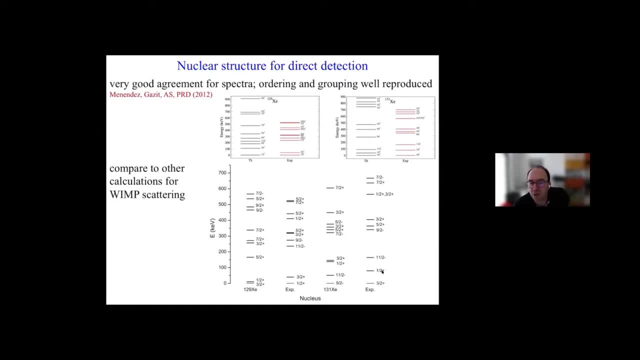 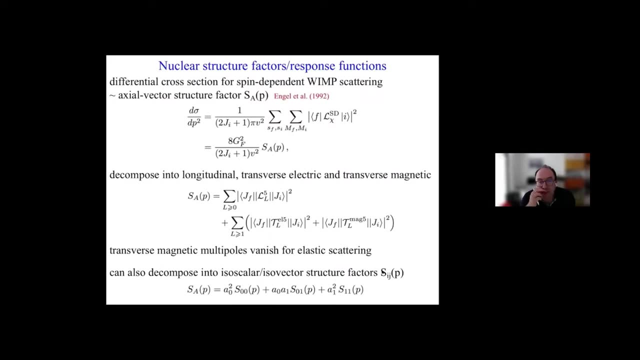 that you have to make sure that your nuclear physics colleagues do before they provide rates for dark matter diode detection. So then we can take these and look first at the nuclear structure factors or the response functions, for this case where the coupling is to the spin. 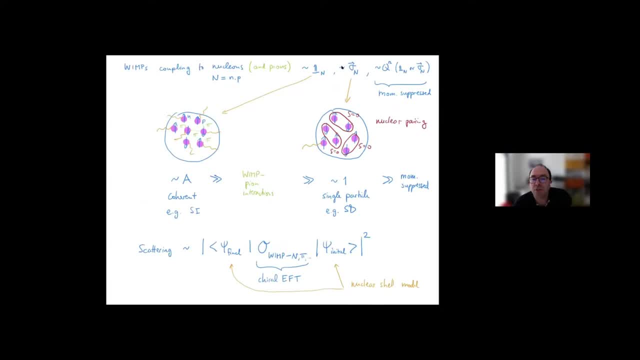 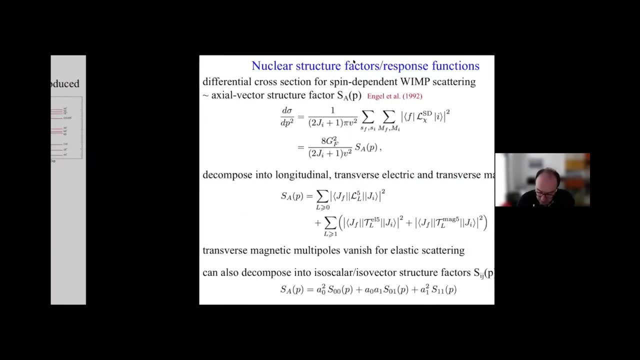 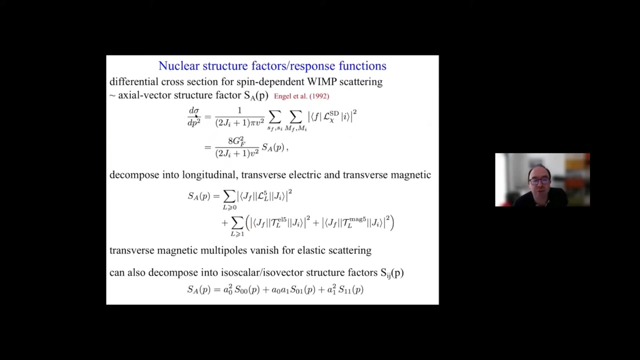 So the coupling has a coefficient that we don't know, because we don't know the WIMP coupling, and it couples to the spin of the nucleon. And then to calculate the cross-section for WIMP, nuclear scattering as a function of the momentum transfer, p squared- we have to go from the initial nucleus. 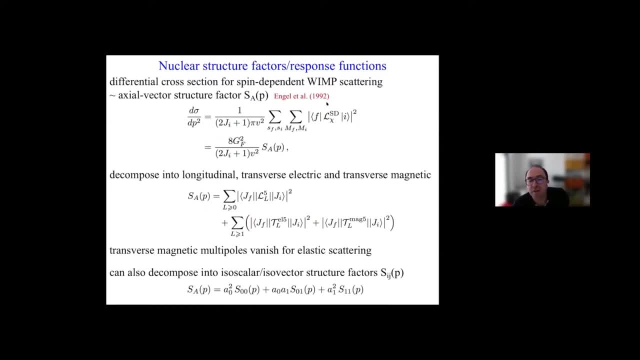 to the final nucleus, which for elastic scattering is the same. There's the interaction operator or Lagrangian in between, And then we have to calculate the cross-section And we can turn all of this into using the standard convention where this involves the coupling of the WIMP to the nucleon. 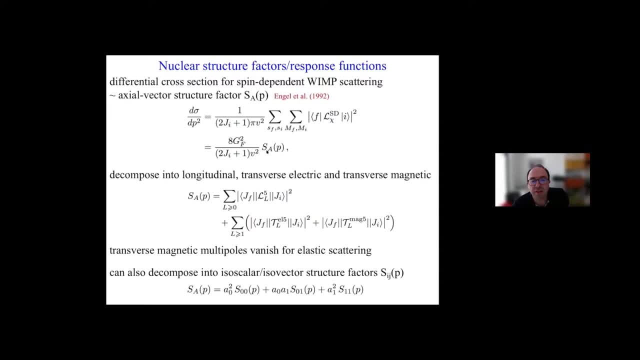 So there's like a single nucleon cross-section times, an axial structure factor, or what is called the structure factor or the response function, which includes all the nuclear structure, physics. And there are various ways to write the nuclear structure factor here, S-A. either we can write it in terms of different multiples. 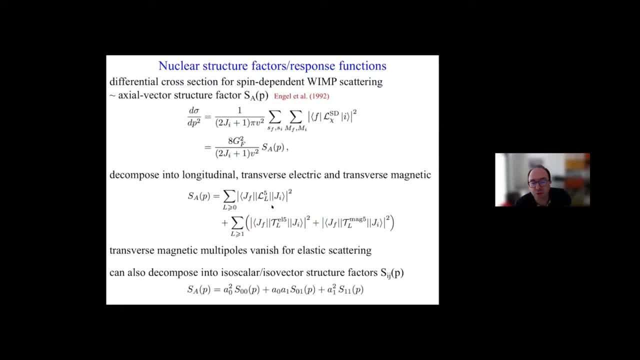 So there's like a multiple expansion. So then it includes basically all the different current operators, Or you can decompose it in isospin. So there's some isoscalar or isovector structure factors. For me, actually, the only thing I'd like to, that we just need. 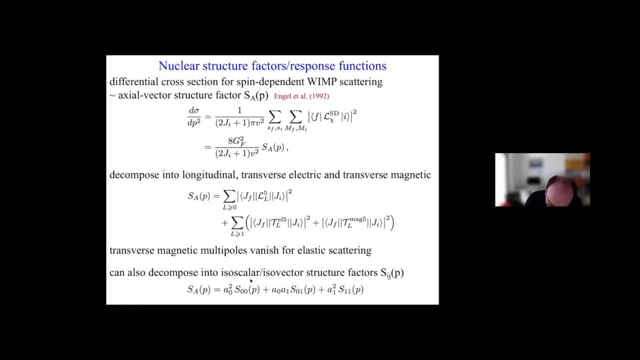 is that we describe basically the cross-section here as, say, a standard single nucleon cross-section sigma where a WIMP happens to a single nucleon times a modification factor S-A, P, which includes all the nuclear physics. 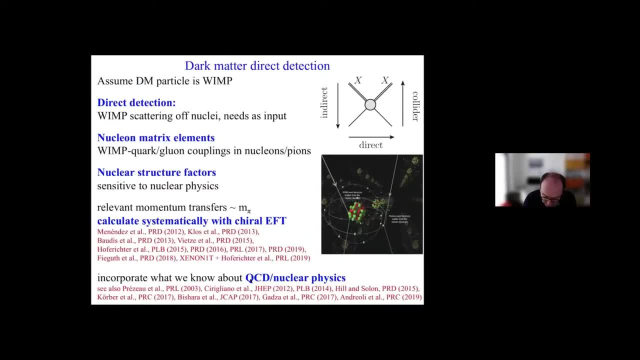 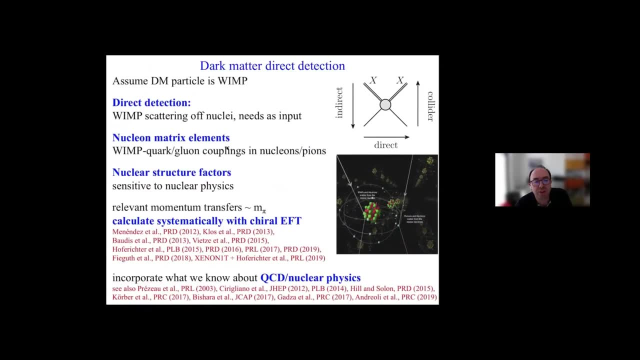 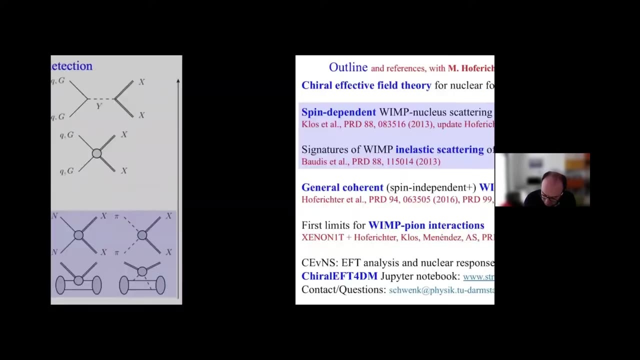 So to keep it in this overview, here this is the single nucleon cross-section, It's basically a nucleon matrix element And the structure factor is the stuff that happens inside the nucleus. Or here there's a matrix element which then defines the single nucleon cross-section. 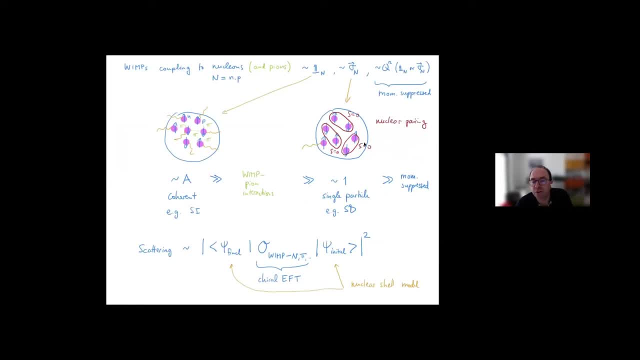 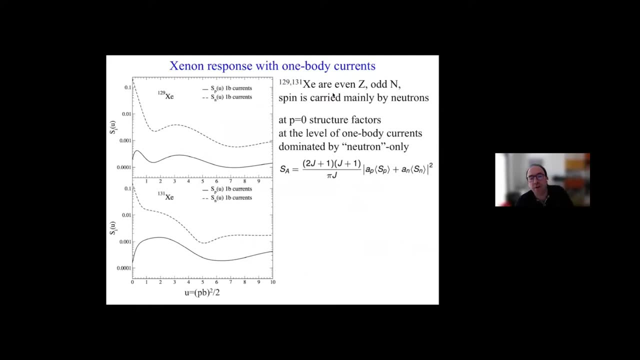 And there's a structure factor that describes all the strong interactions inside the nucleus. OK, And we can calculate this for xenon, And this is for the odd xenon isotopes, because they have even number of protons, So protons are fully paired. 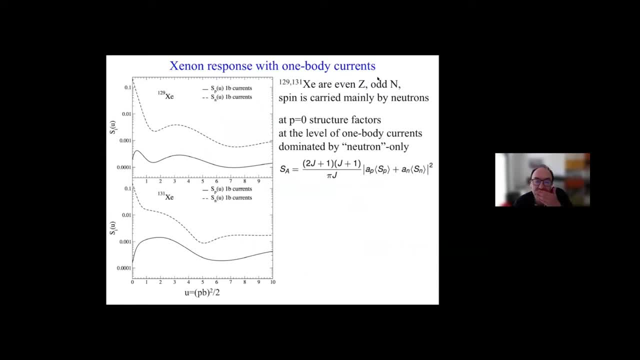 And an odd number of neutrons. So for these xenon isotopes the spin is mainly carried by this free, unpaired neutron And in fact if you look at the response functions as a function of momentum transfer here in some units, then you can see that for xenon 129 and 131,. 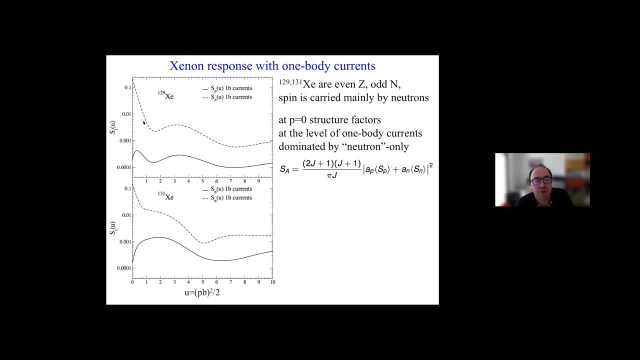 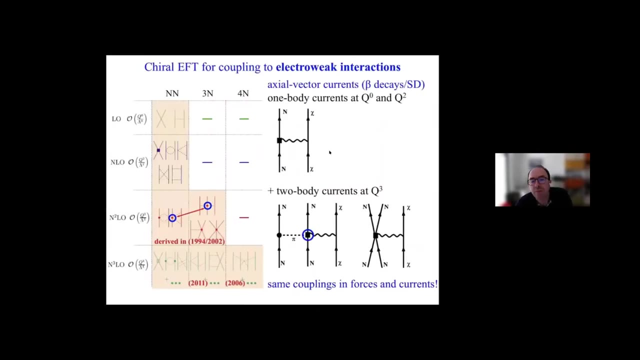 the structure factor is largest for dashed lines, which is the coupling to neutrons And in fact at zero momentum transfer. you can express it as the spin expectation values. But, as I told you, WIMPs don't only have to couple to a single nucleon, but the WIMPs when 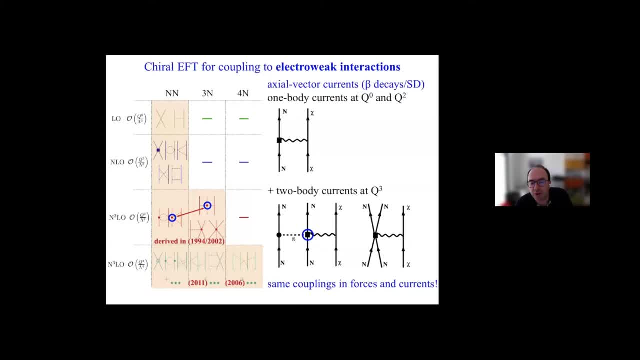 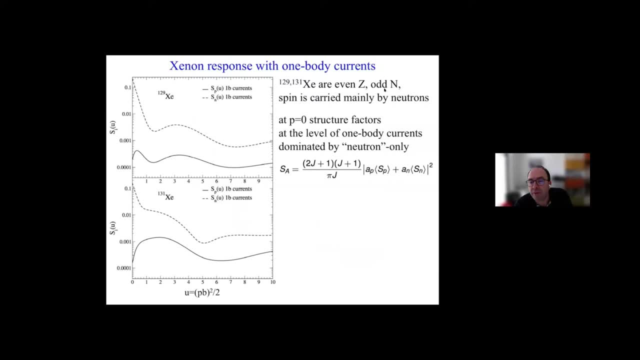 they couple to a nucleon. they don't match up with a single nucleons inside the nucleus. the nucleus also strongly interact and xenon. we have an, the, the unpaired one is a neutron. so the, the large response would here be: this is a neutron. 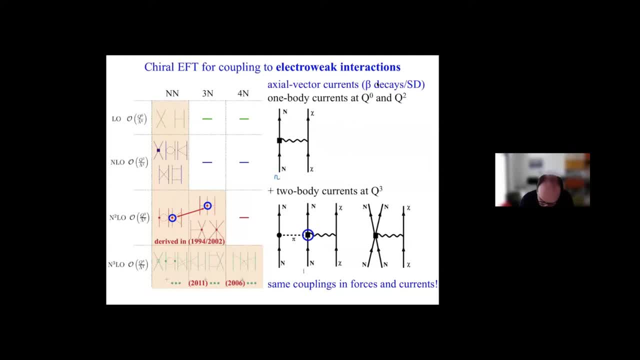 that were the dashed lines before. so one of these has to be a neutron, um, but we can also have a, but we can also have in a nucleus a coupling to two particles. so then we couple to a pair and neutron and a proton. okay. so, while in the case where the single particle coupling is to 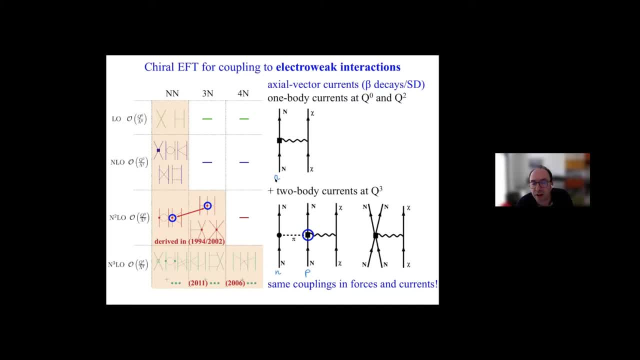 the neutron, the cross already large and in the, when we include these effects where wimps coupled to protons pairs of nucleons, that even if the coupling of wimps is purely to protons, it still talks to the neutrons and talks to the spin unpaired neutron. okay, and this two-body current effect here. 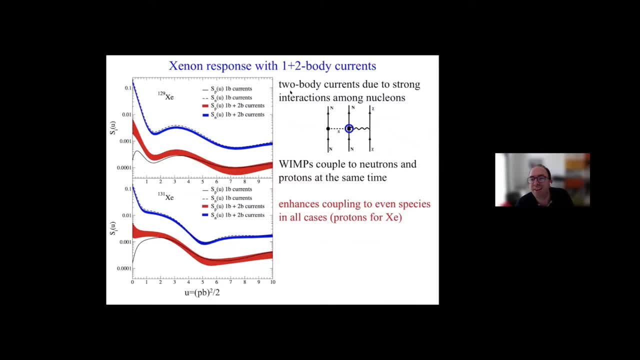 almost done. fedor two-body current effect is something that gives an enhancement at low momentum transfer to the unpaired um to the to the paired species. so you can see that once two body currents are included here with the colored bonds, then even if you assume that the 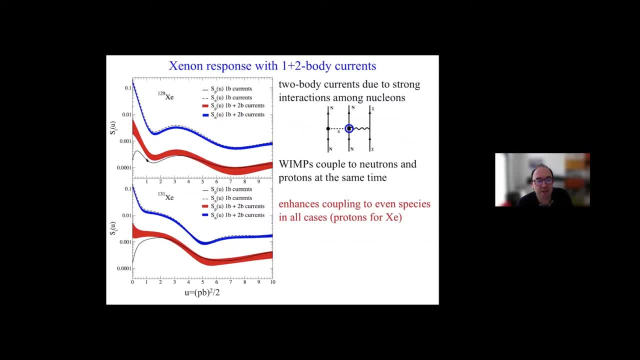 wind couples only to the proton. there's this line here. then then, because of the two body current, because of this coupling- where so, let's say, red is only couples to the proton, then because the other particle can be a neutron, then even though the one body proton coupling is, 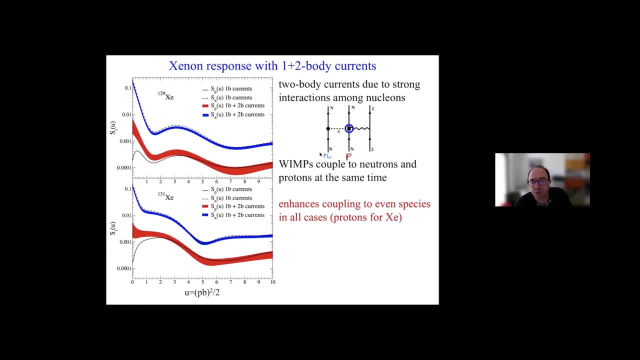 weak the two body. neutron coupling is not proton coupling is proton neutral coupling is not weak because the neutrons still know about the spin expectation value of the non-zero unpaired species. so you can see here that the response of the odd species follows very closely the um, the response of 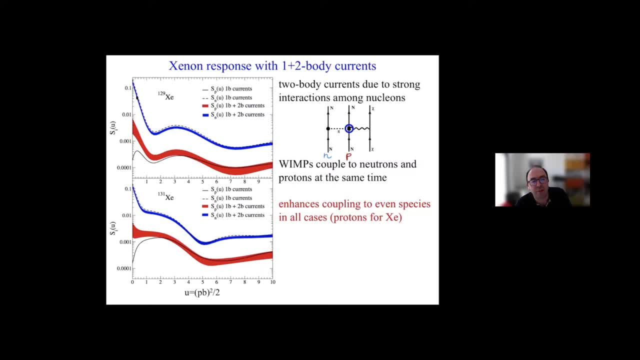 the paired species follows very closely the unpaired. it's just weaker because the one body response is weaker. okay, so this enhances the coupling to the even species, even in the case of, in all cases, in the case of protons, for xenon, and we found this kind of effect in all isotopes. 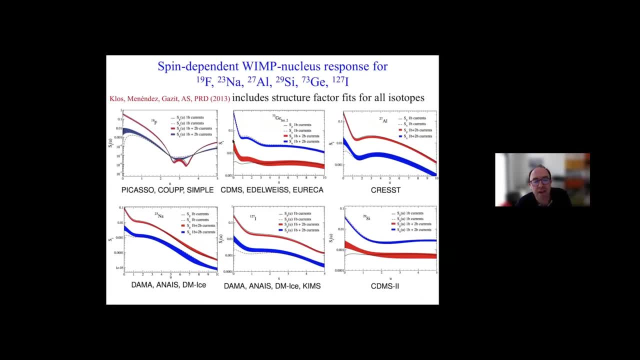 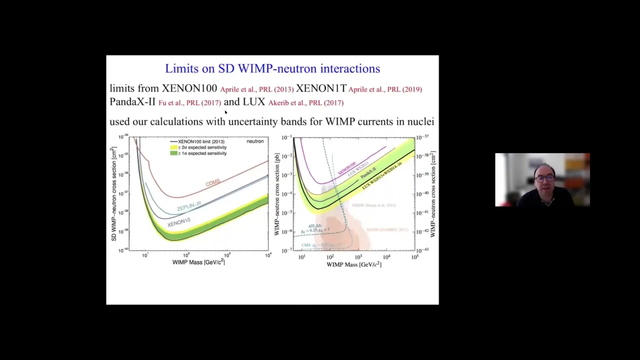 for obvious reasons. so germanium gets enhanced from two body currents, aluminum- aluminum is dominantly protons, but the neutrons get enhanced from two body currents and so forth and um and so um. when we then calculated this and we calculated these for xenon- and we're delighted that the xenon collaboration at that time in the xenon 100 limits- 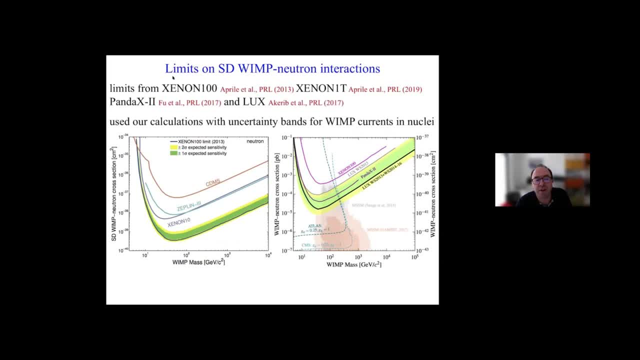 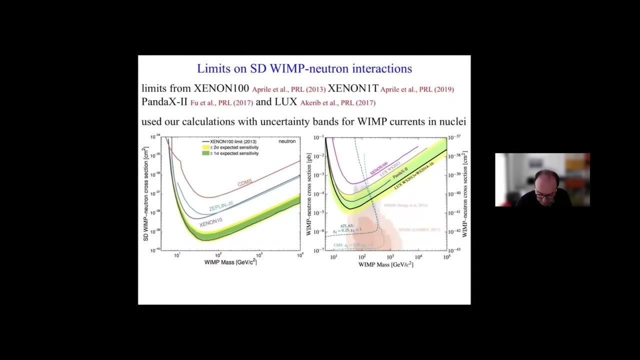 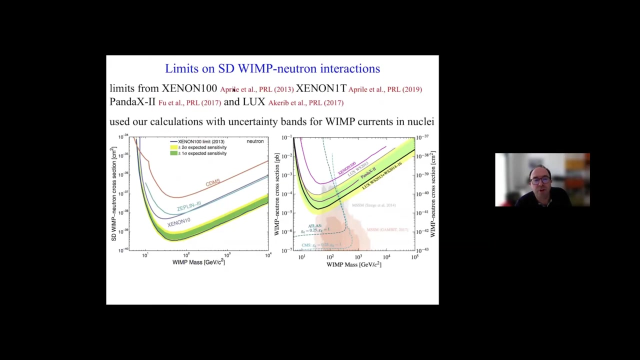 immediately used our structure factors based on these karl aft one and two body currents. and here we can see the back then xenon 100 limit for the wimps coupling to the neutron. so that's the large species, wimps coupling to the neutrons. that's a large species. and also all later with neutron plots were or limits. 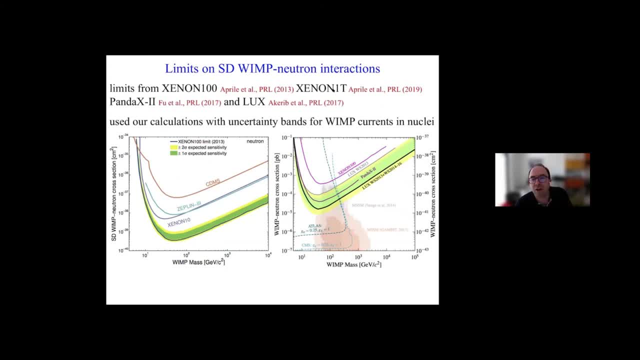 by panda x2, by lux and by xenon, 1 ton used exactly the same structure factor. so this is very important, because one compares this on the same plot. okay, um, so that really was great for us nuclear physicists. um, and then i want to say i shall show you why that's important. if you now look at closely, look at. 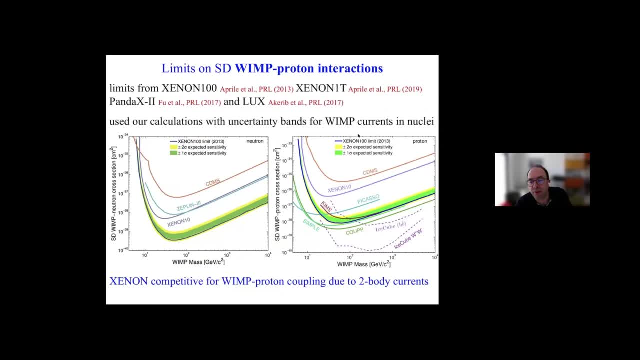 the wimp proton limits. this is from the xenon 100 paper, so you can see that for the wimp neutron limits, xenon 100 improves the sensitivity compared to xenon 10 by an order and a little bit more in cross-section. okay, so one order of magnitude. 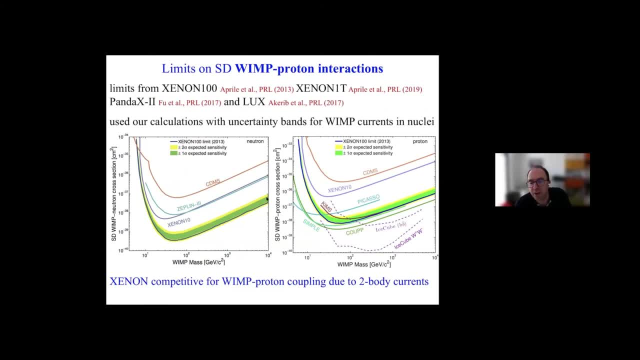 better sensitivity and a little bit more, maybe one and a half orders. however, if you look at the wimp proton limits from the same experiment, going from xenon 10 to xenon 100, the order of improvement is almost two orders of magnitude. and this improved sensitivity is not because there was something. 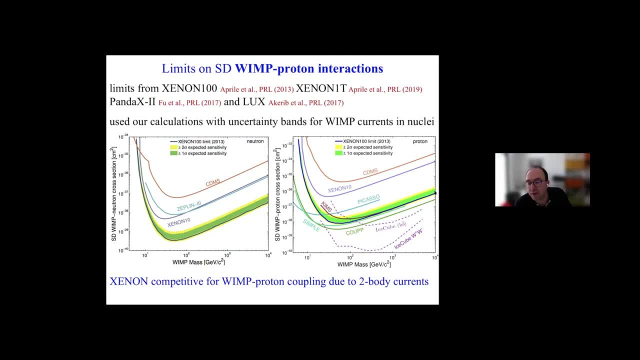 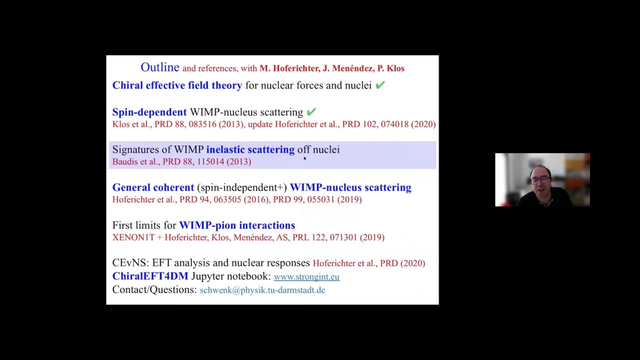 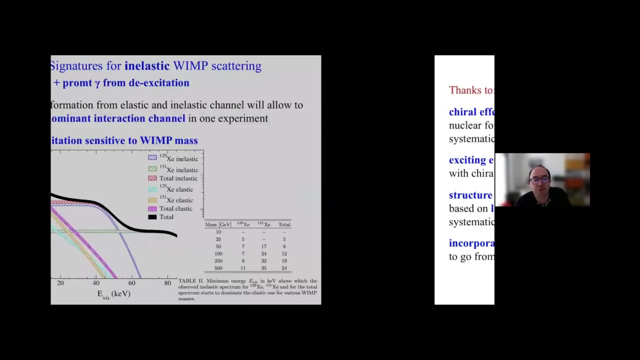 special about the protons. it's because of this enhancement from the two body currents that the xenon experiment now becomes also competitive to win proton couplings. okay, and with this i will check off this and leave this part for inelastic scattering for tomorrow and um, just keep you here the summary, with thanks to collaborators. 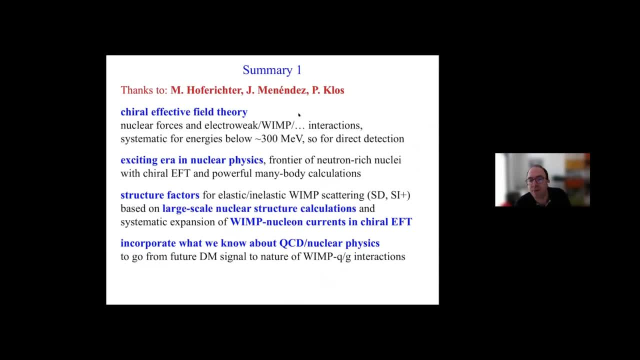 and maybe leave this for you to read so that i don't take too much more time. thank you very much for um coming and i hope you have questions and look forward to the exercises later. 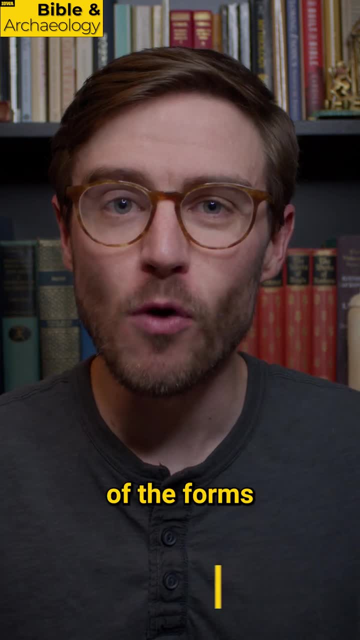 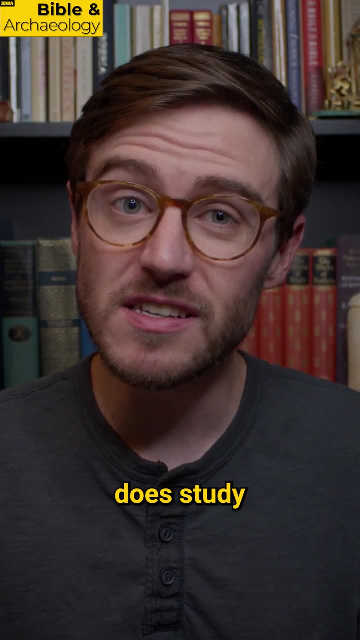 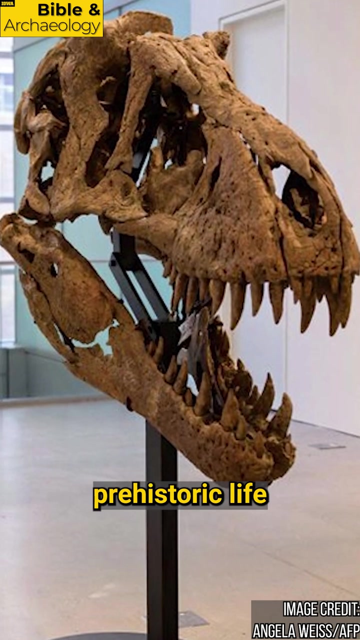 What is paleontology? Paleontology is the study of the forms of pre-existing life as represented by the fossils of plants, animals and other organisms. While archaeology does study the relationships and interactions between human and animal life, archaeology does not include the study of non-human prehistoric life that existed before the earliest humans. 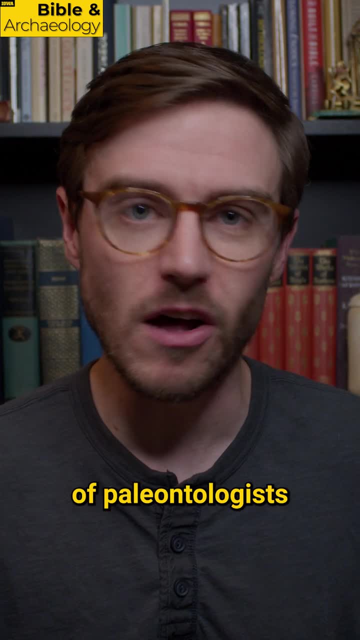 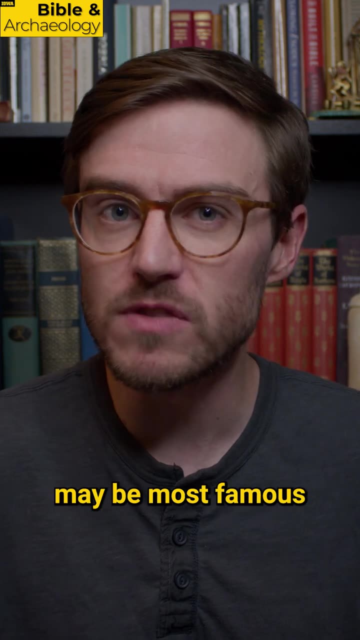 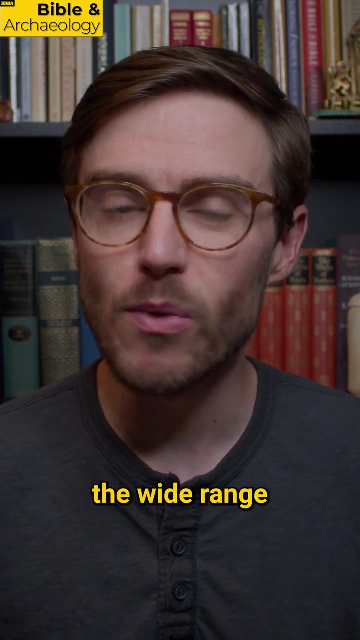 like dinosaurs. This area of study is the domain of paleontologists, who specialize in studying and understanding these life forms in the fossil record. While paleontology may be most famous for studying fossilized dinosaur bones, paleontologists can specialize in several sub-disciplines which cover the wide range of fossilized remains, including 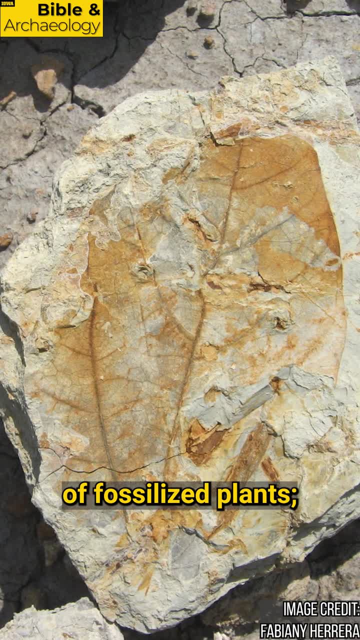 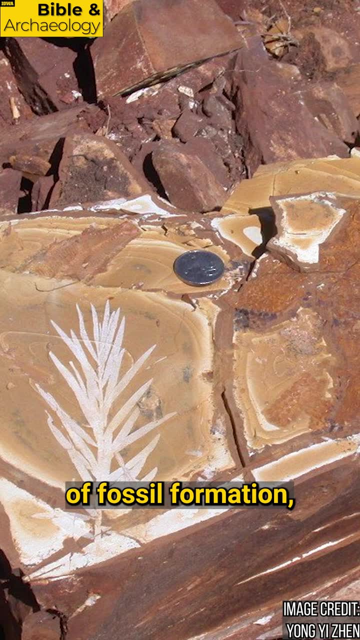 specializations like paleobotany or the study of fossilized plants, palynology, the study of pollen and spores, and taphonomy, the study of the processes of fossil formation, decay and preservation. For all of us here at Bible and Archaeology, I'm Jordan James. I'll see you next time. 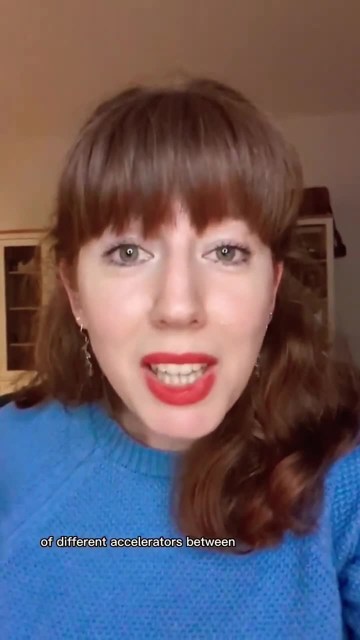 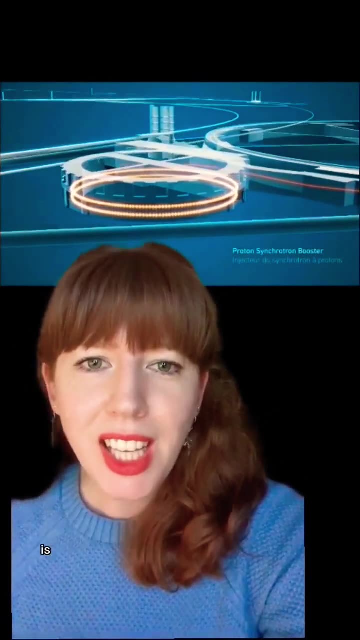 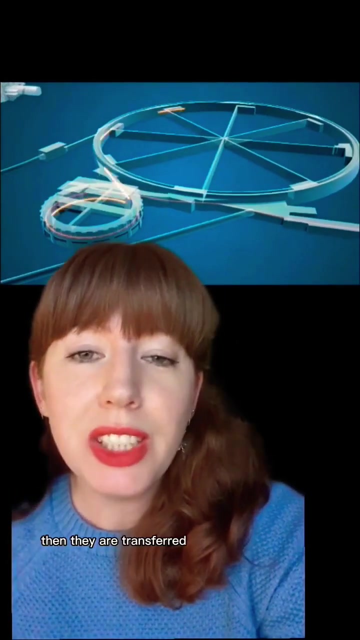 But then we go through a number of different accelerators between the LINAC and the LHC. Let's follow the protons journey. The first circular accelerator that protons see is the proton synchrotron booster, and this accelerates the protons to 2 GeV. Then they are transferred into the proton synchrotron.